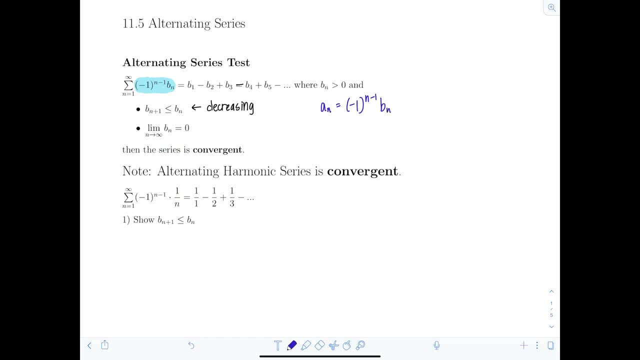 it doesn't matter, just some sort of alternating series. And if you take out the alternating part, that's the sequence bn. So bn basically equals the absolute value of a sub n. all right, And if these two conditions are the same, then we have b sub n minus 1 to the n minus 1 times bn. 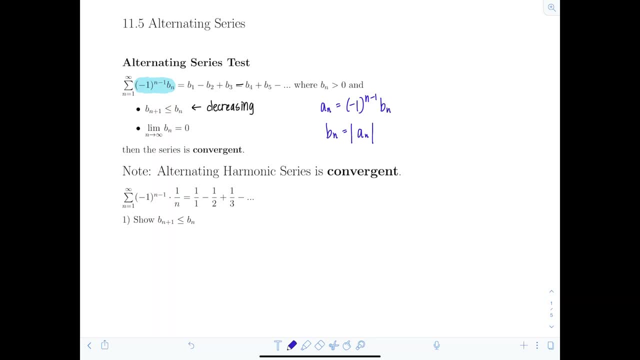 and if these two conditions are satisfied, then according to the alternating series test we can say our original series, the sum of an, is convergent. If either condition fails, then the alternating series test does not apply and then you're going to have to discuss the 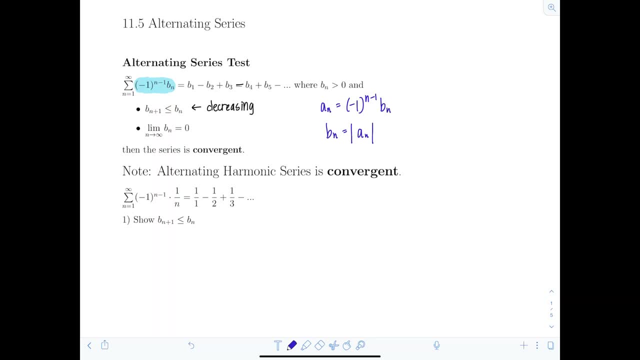 convergence or divergence some other way. So, as a note, the alternating harmonic series is convergent. So the alternating harmonic series is the sum n equals 1 to infinity, of negative, 1 to the n minus 1 times bn. So if the alternating harmonic series is convergent, then the sum n equals 1 to. 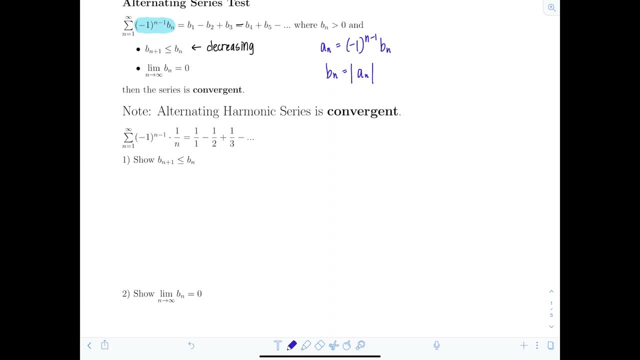 the n minus 1 times 1 over n. And notice, our original harmonic series just consists of the sum n equals 1 to infinity of 1 over n. but the alternating harmonic series is the harmonic series in which the terms alternate. So let me list out for you a sub n for the alternating harmonic. 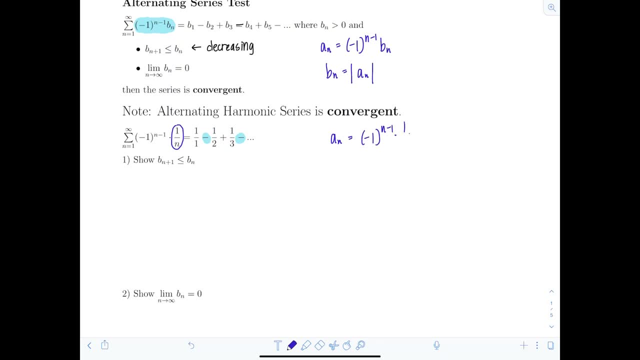 series is negative 1 to the n minus 1 times 1 over n, and that means b sub n. the absolute value of a sub n would just be negative: 1 to the n minus 1 times 1 over n. So if the alternating harmonic series is convergent, then the sum n equals 1 to infinity of 1 times 1 times 1 over n. So if the alternating harmonic series is convergent, then the sum n equals 1 to infinity of 1 times 1 times 1 over n. You can: 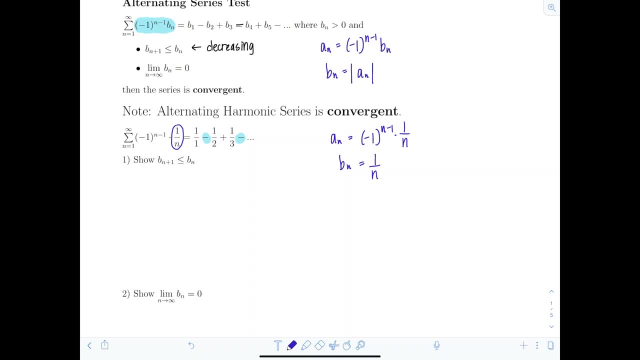 just take off that negative 1 to the n minus 1 or negative 1 to whatever power part. Okay, so I'm going to apply the alternating series test now to the alternating harmonic series and show that it's convergent. First thing I need to show is that it's decreasing. So b sub n plus 1. 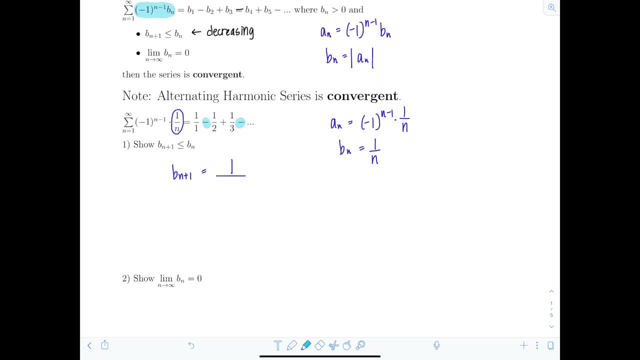 is equal to 1 over. well, I'm just going to substitute n plus 1 here, n plus 1.. And if I compare that to 1 over n right, which is b sub n, clearly now the denominator is larger. So that whole. 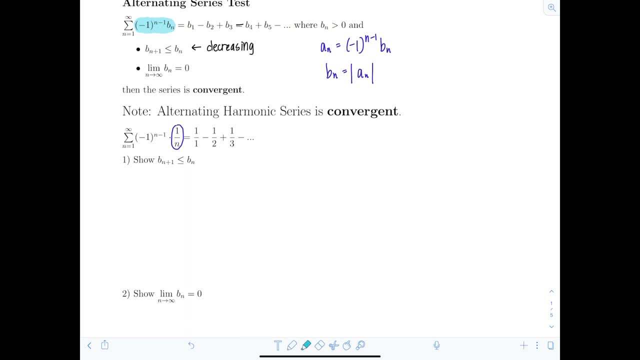 infinity of 1 over n. but the alternating harmonic series is the harmonic series in which the terms alternate. So let me list out for you. a sub n for the alternating harmonic series is negative, 1 to the n, minus 1 times 1 over n, and that means b sub n. the absolute value of a sub n would just be 1. 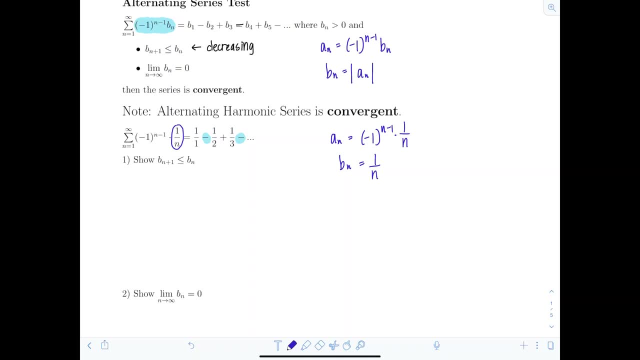 over n. You can just take off that negative 1 to the n minus 1 or negative 1 to whatever power part. Okay, so I'm going to apply the alternating series test now to the alternating harmonic series and show that it's convergent. First thing I need to show is that it's decreasing. 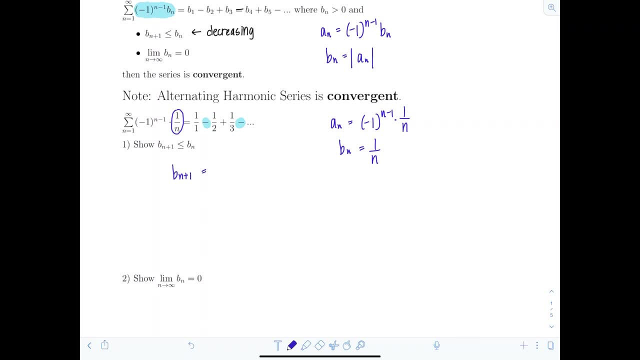 So b sub n plus 1 is equal to 1 over 1.. So I'm just going to substitute n plus 1 here n plus 1.. And if I compare that to 1 over n right, which is b sub n, clearly now the denominator is larger, So that whole expression. 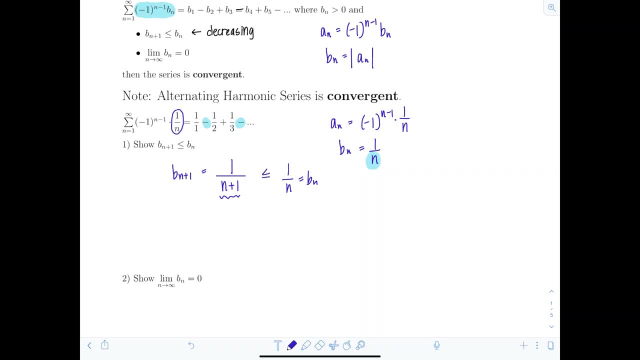 b sub n plus 1 is going to be less than or equal to 1 over n. So the first condition is satisfied. Then condition 2, I need to show that the limit, as n approaches infinity, of b sub n is 0.. 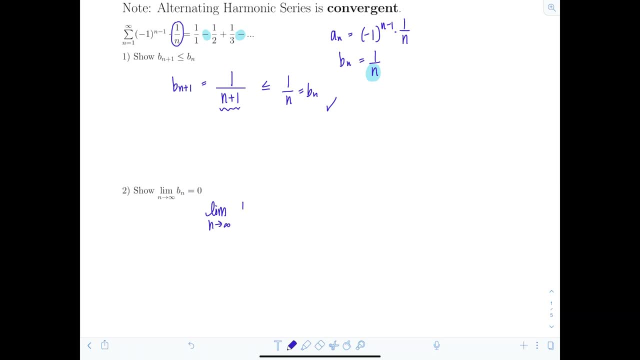 So the limit is 1 over n. As n approaches infinity, of 1 over n, well, that's clearly 0. So both conditions have been satisfied. So this implies always write the original series. so the sum n equals 1 to infinity. 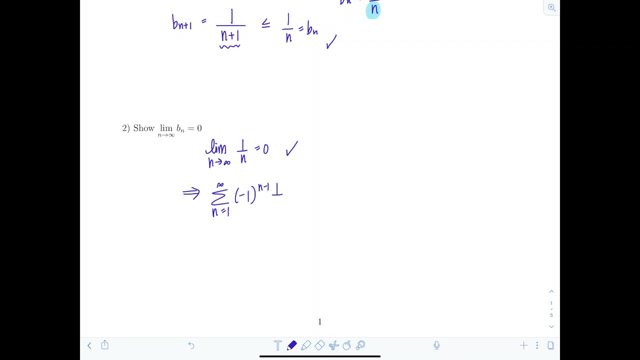 of negative 1 to the n minus 1 times 1 over n. That converges by the alternating series test: All right, And that's our final answer. One more go Beautiful, All right. Now, remember the original harmonic series was divergent. 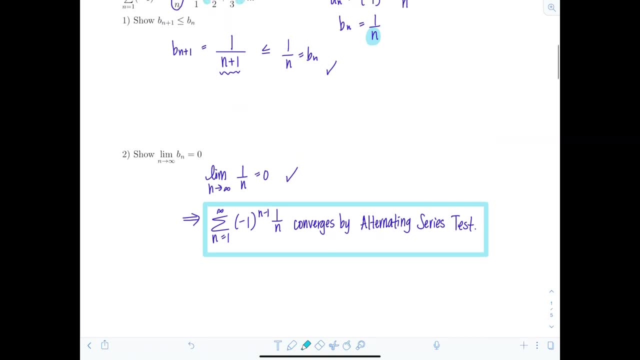 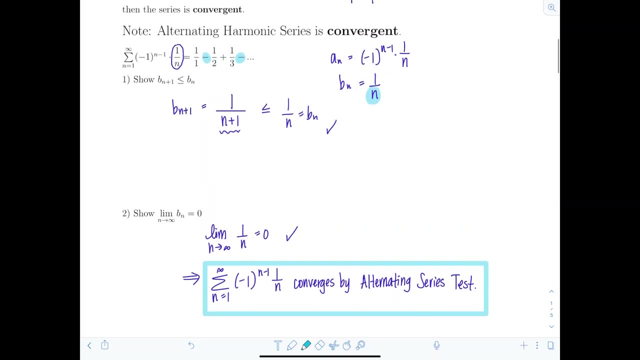 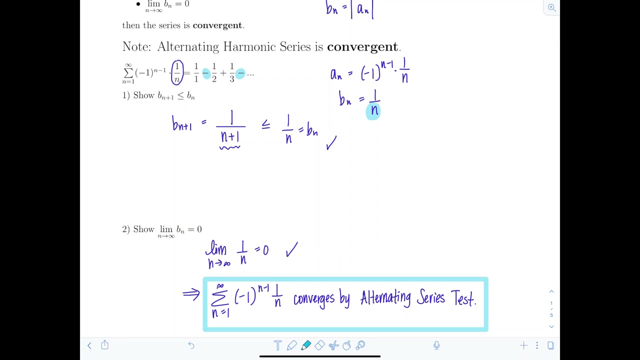 And we talked about the fact that the terms were decreasing, but they weren't decreasing fast enough so that the infinite sum converged. And why does the alternating series test converge? Well, look at what's happening. Because every other term, if the term, is negative, then that's going to cause the series or the sum of the terms to shrink more quickly. 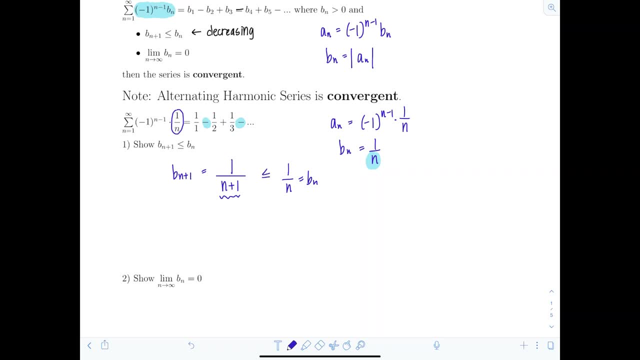 expression b sub n plus 1 is going to be less than or equal to 1 over n. So the first condition satisfied. Then condition two: I need to show that the limit as n approaches infinity of b sub n is zero. So the limit as n approaches infinity of 1 over n, well, that's clearly zero. So both 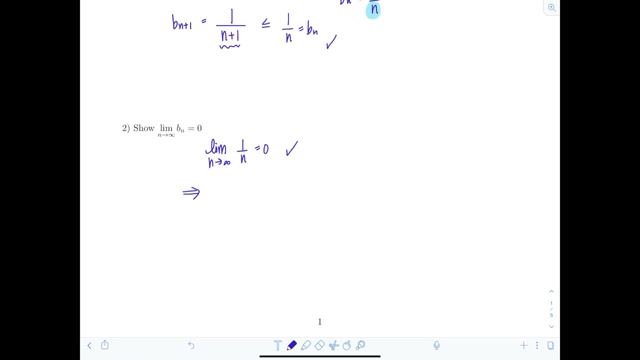 conditions have been satisfied. So this implies always write the original series. So the sum n equals 1 to infinity of negative, 1 to the n minus 1 times 1 over n. That converges by the alternating series test. All right, and that's. 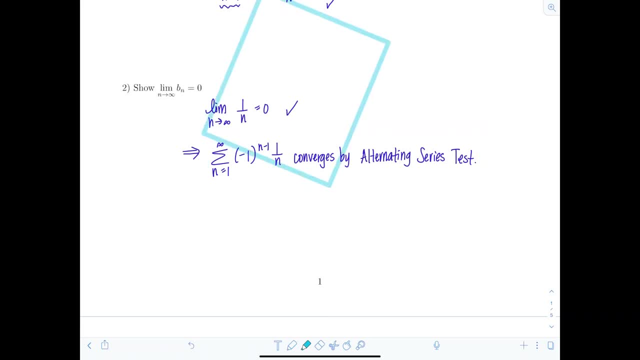 our final answer? Oops, One more go Beautiful, All right Now remember the original harmonic series was divergent And we talked about the fact that the terms were decreasing, but they weren't decreasing fast enough so that the infinite sum converged. And why does the alternating series test converge? 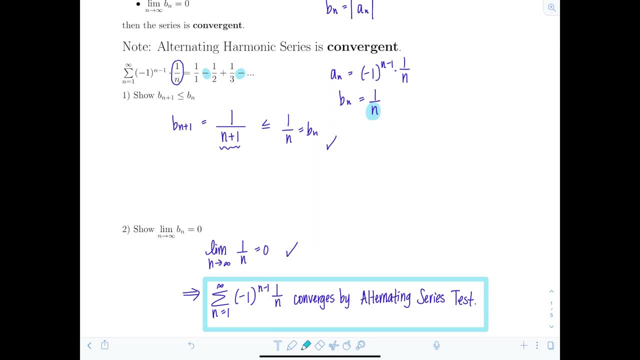 Well, look at what's happening, Because every other term is negative, then that's going to cause the series, or the sum of the terms, to shrink more quickly, And so that's why the alternating harmonic series converges, whereas the regular harmonic series diverges. 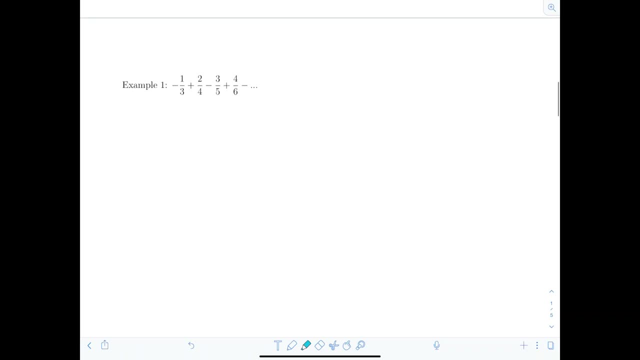 All right, let's get into some more exciting examples. So example one: Here we have the following series: negative: 1 3rd plus 2 4ths, minus 3 5ths plus 4 6ths. The fractions haven't been. 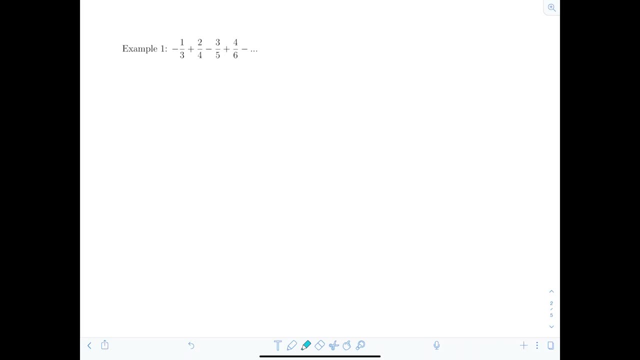 reduced in order to help us identify a pattern, because we have to express this series first in summation notation using sigma notation, So I can write it as the sum of the terms Sum. It seems like the most natural place to start would be with n equals 1.. And then in the 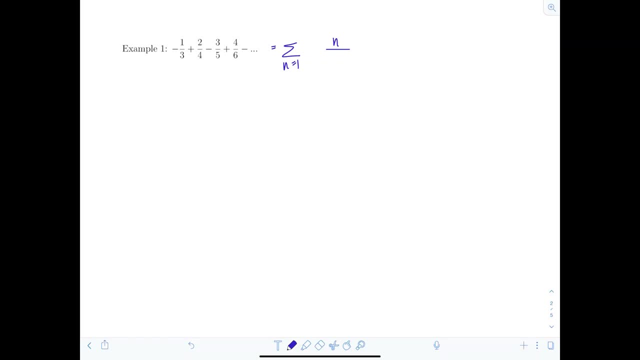 numerator. I would just have n right And then notice the denominator is always 2 greater than the numerator. So if I have n in the numerator, then I would have n plus 2 in the denominator. So sum n equals 1 to infinity, And then I'm going to have negative 1.. Now I have to 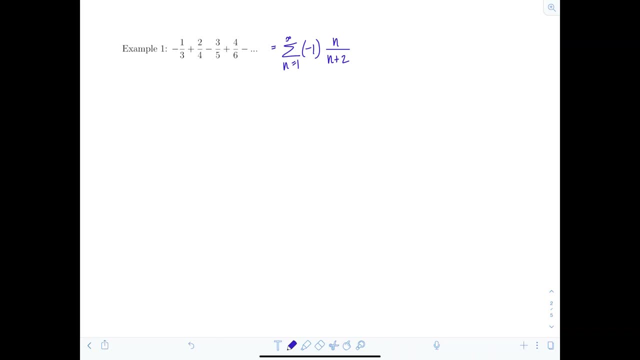 determine if it's going to be raised to the nth power or to the n minus 1 or n plus 1.. So just decide: Is the first term needing to be positive or negative? Well, the first term is negative, so negative. 1 should be raised to the nth power, since. 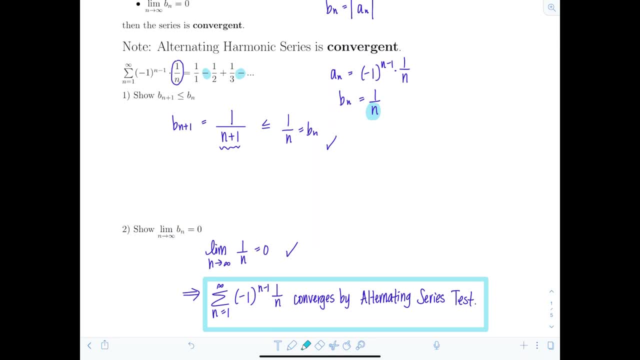 And so that's why the alternating harmonic series converges, whereas the regular harmonic series diverges. All right, Let's get into some more exciting examples. So example one: here we have the following series: negative 1. third plus 2 fourths minus 3 fifths plus 4 sixths. 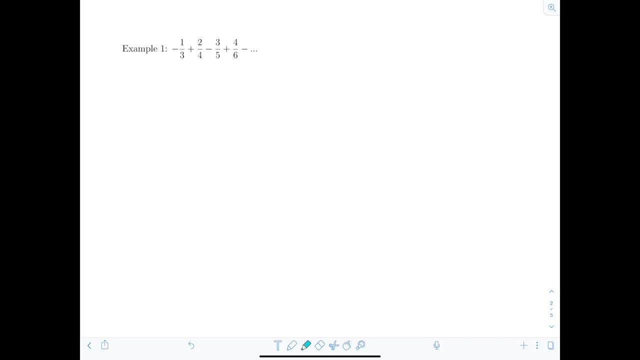 The fractions haven't been reduced in order to help us identify a pattern, because we have to. you know, we're going to have to go back and forth between them Because we have to express this series first in summation notation using sigma notation. 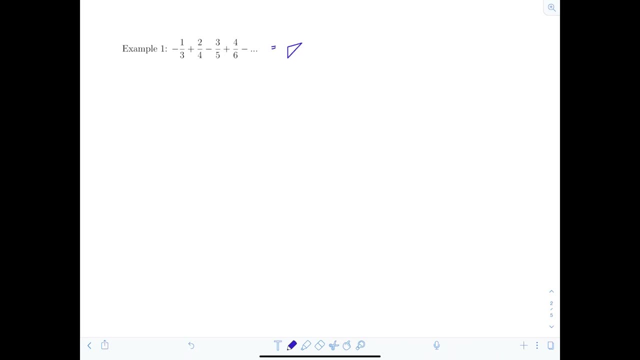 So I can write it as the sum. It seems like the most natural place to start would be with n equals 1.. And then in the numerator I would just have n right, And then notice the denominator is always 2 greater than the numerator. So if I have n in the numerator, then I would have n plus 2 in the denominator. 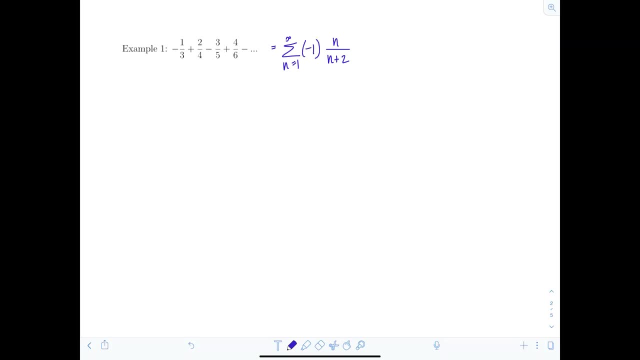 So sum n equals 1 to infinity, And then I'm going to have negative 1.. Now I have to determine if it's going to be raised to the nth power or to the n minus 1 or n plus 1.. So just decide. is the first term needing to be positive or negative? 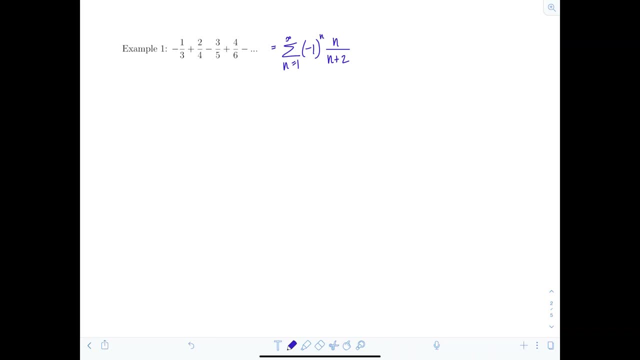 Well, the first term is negative, So negative 1 should be raised to the nth power, since we're starting at 1, right, Then I would have negative 1 to the first and I want that first term to be negative, All right. So this whole expression here is a sub n. Negative 1 to the n. 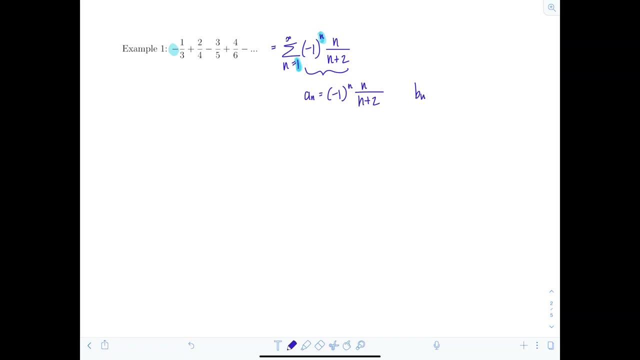 times n over n plus 2. That means b sub n. what we're going to focus on right now, when we apply the AST alternating series test, is just n over n plus 2.. Okay, so let's consider the two conditions or two criteria. So first, 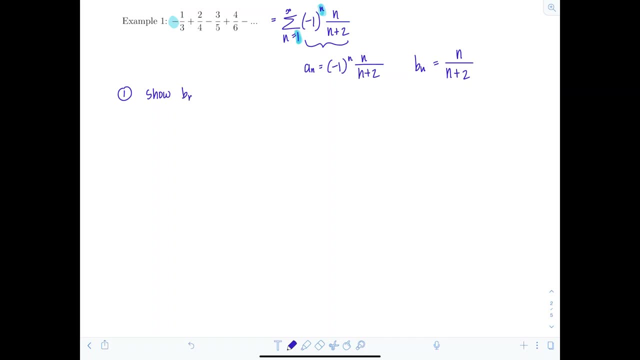 I need to show that b sub n plus 1 is less than or equal to b sub n. Well, let's see What is b sub n plus 1?. Well, that would be n plus 1 in the numerator over n plus 1 plus 2, which is n plus 3 in the denominator. 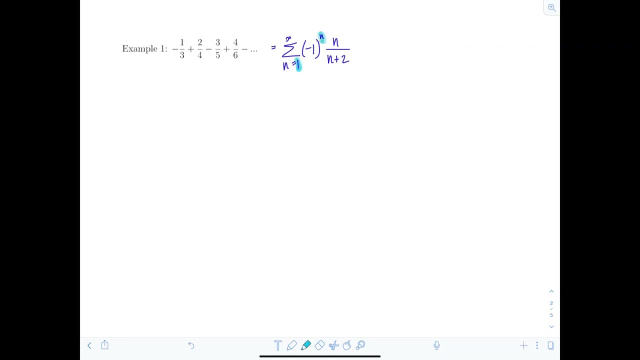 we're starting at 1, right, Then I would have negative 1 to the first and I want that first term to be negative, All right. so this whole expression here is a sub n negative 1 to the n times n over. 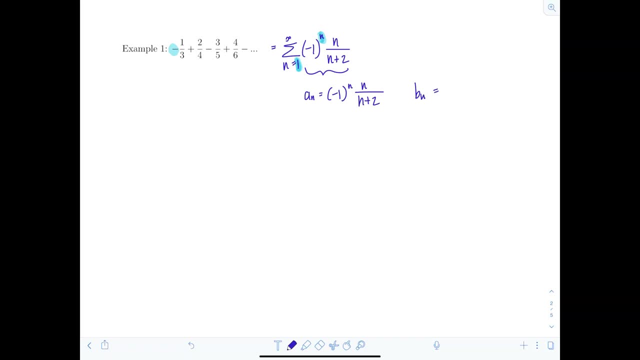 n plus 2. That means b sub n. what we're going to focus on right now, when we apply the AST alternating series test, is just n over n plus 2.. Okay, so let's consider the two conditions or two criteria. 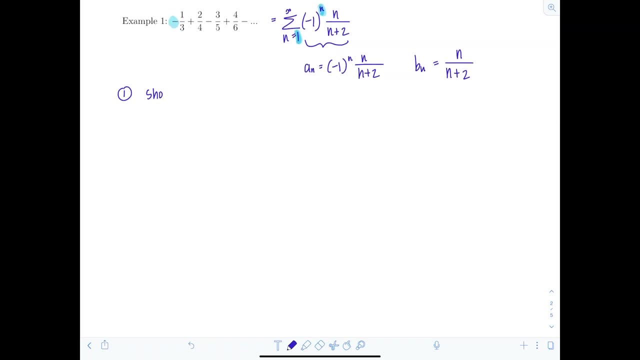 So first I need to show that b sub n plus 1 is less than or equal to b sub n. Well, let's see what is b sub n plus 1? Well, that would be n plus 1 in the numerator over n plus 1 plus 2, which is n plus 3 in. 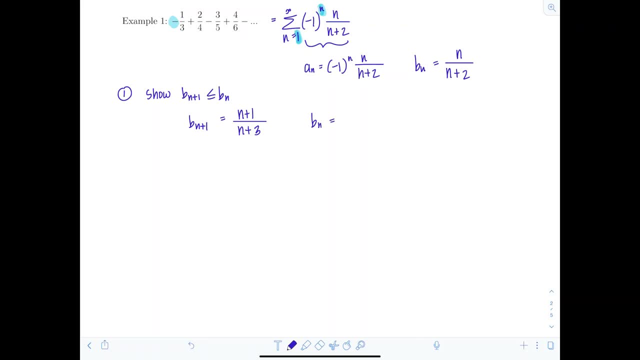 the denominator, And b sub n is n over n, n plus 2.. Now, in this case it's not clear. I can't obviously show inequality one way or another because, notice, the numerator increased and the denominator increased, So this is not an obvious inequality, the way it was when we were considering the alternating. 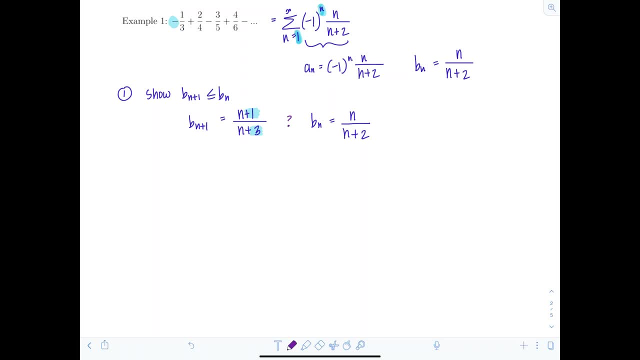 harmonic series in the previous example. So when this comes up, what you want to do is use our other definition for decreasing, and that has to do with derivatives. But remember, we can't differentiate a sequence, So I have to first define a function. 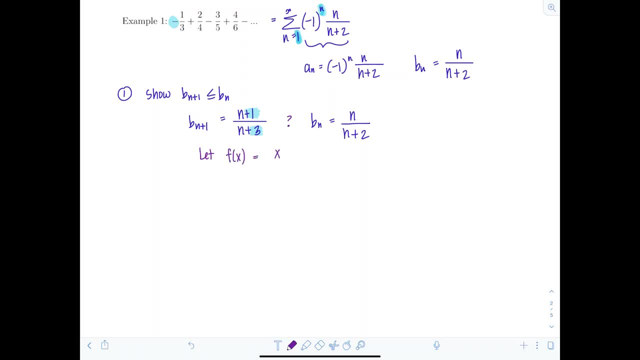 I'm going to let f of x equal, x over x plus 2.. And then now I'm going to find f prime of x and see if I can determine whether or not this function is decreasing. So f prime of x, let's apply the quotient rule. 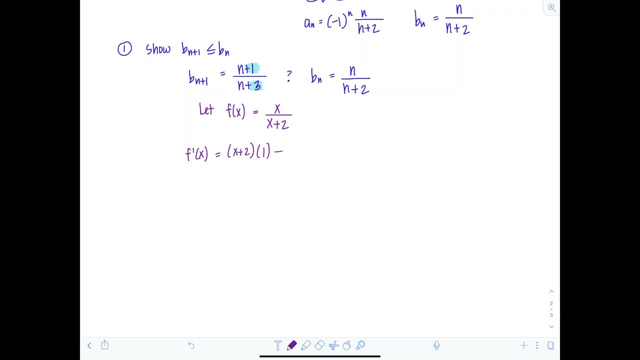 I'm going to have x plus 2 times 1 minus x times 1 over x plus 2 squared, And so in the numerator I just have x plus 2 minus x over x plus 2 squared. So now notice x's cancel out. 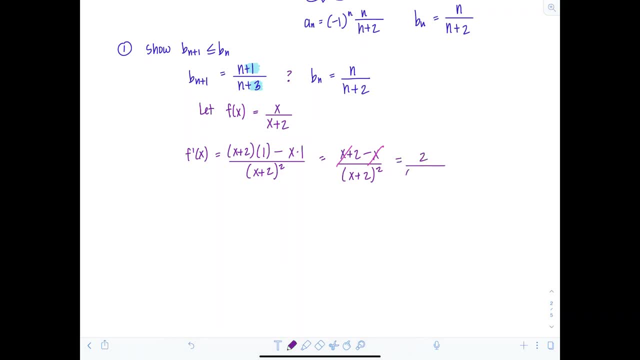 All I'm left with is 2 over x plus 2 squared, And the numerator is positive right, It's a constant 2.. The denominator is some quantity squared, So that's never going to be negative. So in fact, f prime of x is strictly greater than 0.. 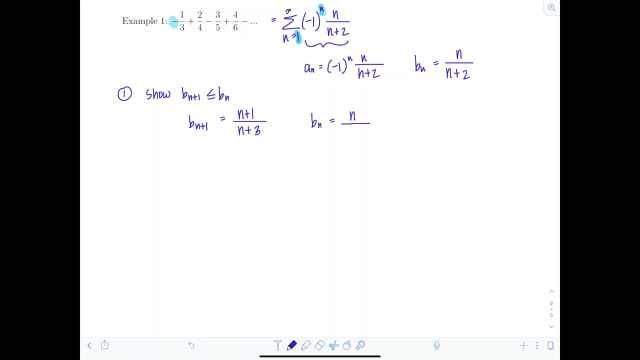 And b sub n is n over n plus 2.. Now, in this case it's not clear. I can't obviously show inequality one way or another because- notice, the numerator increased and the denominator increased, So this is not an obvious inequality, the way it was when we were considering the alternating harmonic series in the previous example. 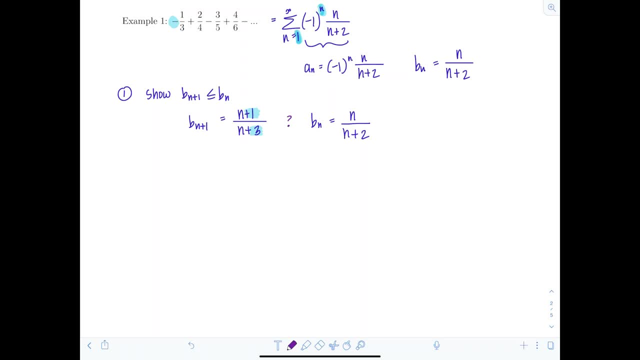 So when this comes up, what you want to do is use our other definition for decreasing, and that has to do with derivatives. But remember, we can't differentiate a sequence, So I have to first define a function. I'm going to let f of x. 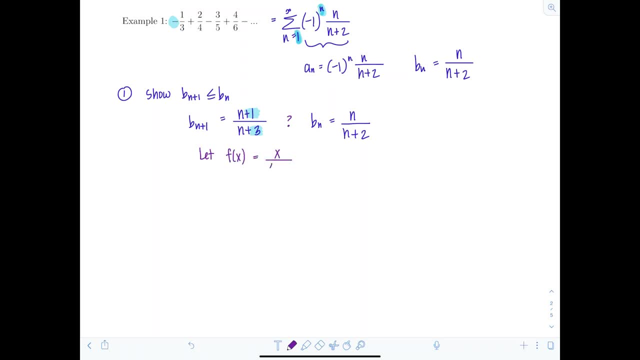 equal x over x plus 2.. And then now I'm going to find f prime of x and see if I can determine whether or not this function is decreasing. So f prime of x, let's apply the quotient rule. I'm going to have x plus 2. 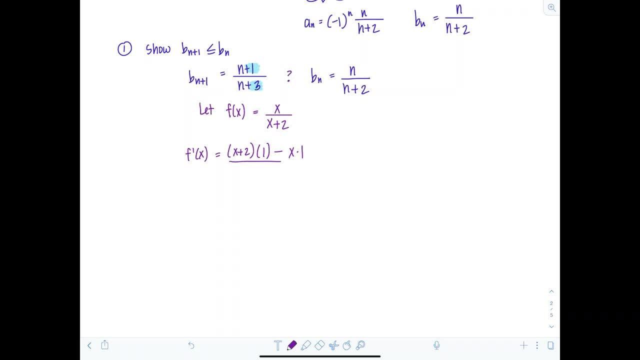 times 1.. Minus x times 1 over x plus 2 squared. And so in the numerator I just have x plus 2 minus x over x plus 2 squared. So now notice x's cancel out. All I'm left with is 2 over. 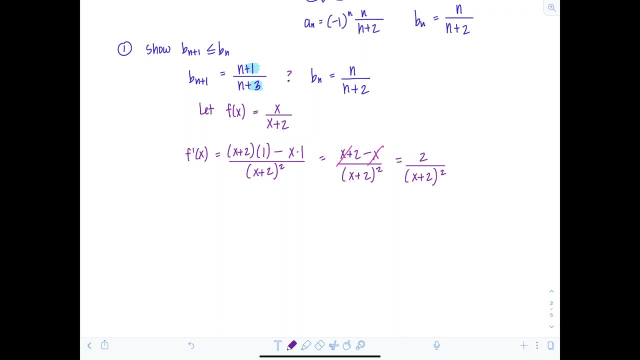 x plus 2 squared And the numerator is positive right, It's a constant 2.. The denominator is positive. The denominator is some quantity squared, so that's never going to be negative. So in fact, f prime of x is strictly greater than 0.. 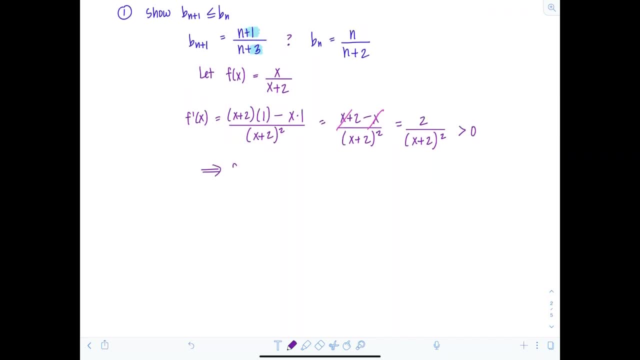 Well, what does that mean? This implies that f of x, our function, is an increasing function, Right? If the derivative is positive, then that means the function's increasing, which means that b sub n plus 1 in my sequence, is actually greater than b sub n. 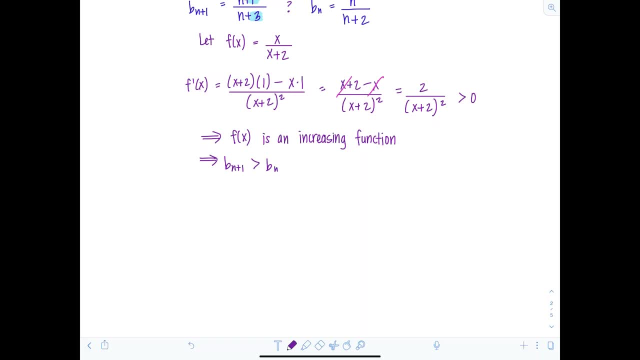 It's an increasing sequence. Well, that's exactly what I'm not trying to show. This means condition 1 fails, So the alternating series test does not apply. What do we do now? Well, you have to apply some other test. 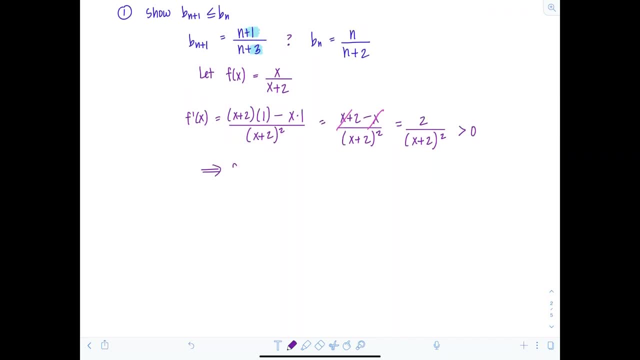 Well, what does that mean? This implies that f of x, our function, is an increasing function, Right? If the derivative is positive, then that means the function's increasing, which means that b sub n plus 1 in my sequence, is actually greater than b sub n. 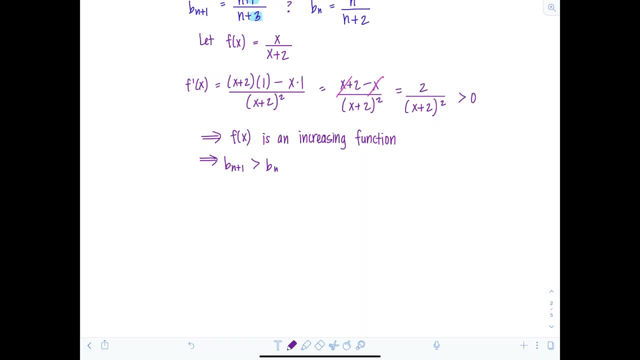 It's an increasing sequence. Well, that's exactly what I'm not trying to show. This means condition one fails, So the alternating series test does not apply. What do we do now? Well, you have to apply some other test And typically, when one of the conditions of the alternating series test fails, 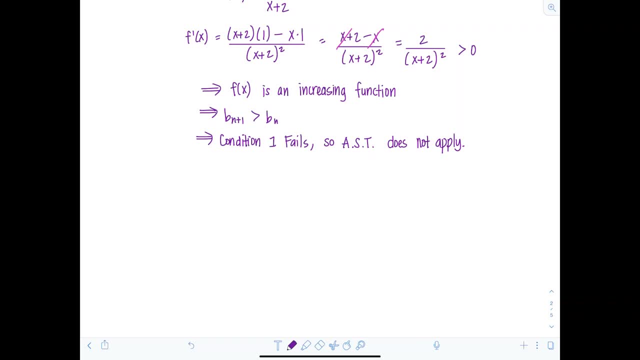 you can just go to the test for divergence and that should help you out. So, in fact, notice The limit as n approaches infinity of a sub n, which is the limit as n approaches infinity of negative 1 to the n times n over n plus 2, does not exist. 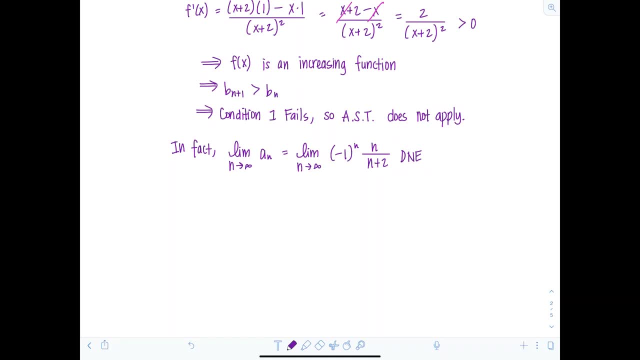 Why can we say that? Well, notice here, since it's alternating, we have the even terms approaching one value for the limit and the odd terms approaching another value. So I'm going to go into a little more detail than probably what's necessary for you. 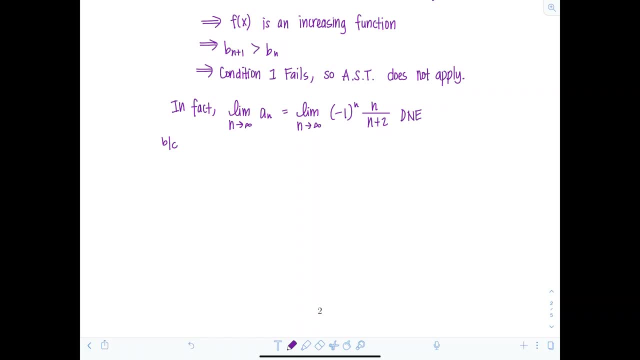 just to demonstrate for this first example, and then from here on out, I'll just kind of cut to the chase when we're working these examples. So here's why. So consider the even terms- Okay, Those I'm going to look at the limit, as n approaches infinity, of all of the even terms of our sequence: a sub n. 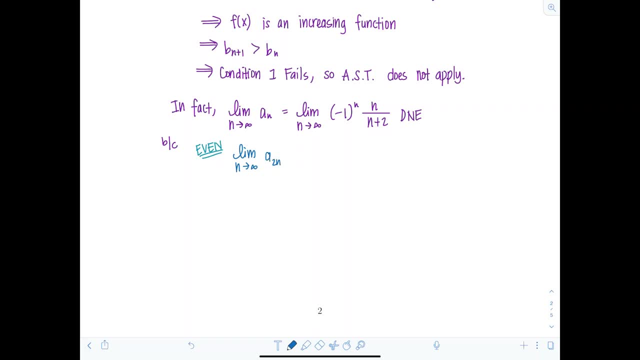 So those would all be The ones with index 2n, right? So this would be the limit, as n approaches infinity, of negative 1 to the 2n times 2n over 2n plus 2.. But negative 1 to the 2n, that's going to be negative 1 raised to an even power. 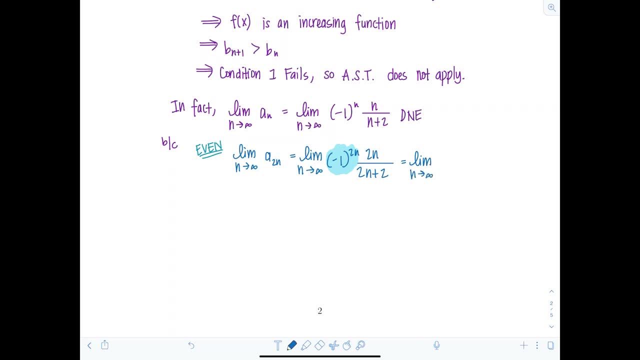 so it's just going to turn into positive 1, times 2n, over 2n plus 2.. And then now, when we take this limit limit, since the degree of the numerator is equal to the degree of the denominator, I can just take: 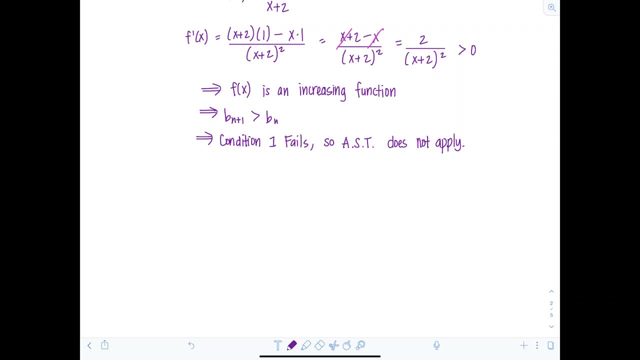 And typically, when one of the conditions of the alternating series test is not applied, you can just go to the test for divergence, and that should help you out. So, in fact, notice the limit as n approaches infinity of a sub n, which is the limit as n approaches infinity of negative 1 to the n. 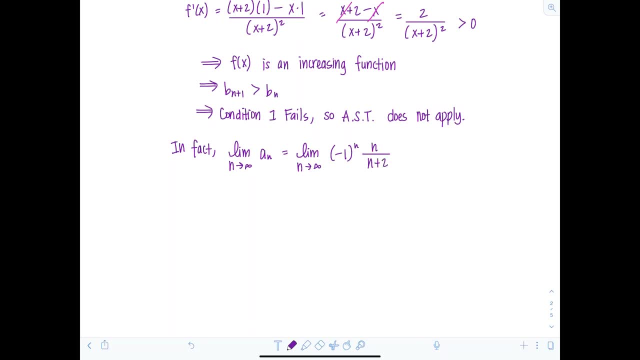 times n over n plus 2 does not exist. Why can we say that? Well, notice that the limit as n approaches infinity of a sub n does not exist. Notice here, since it's alternating, we have the even terms approaching one value for the limit. 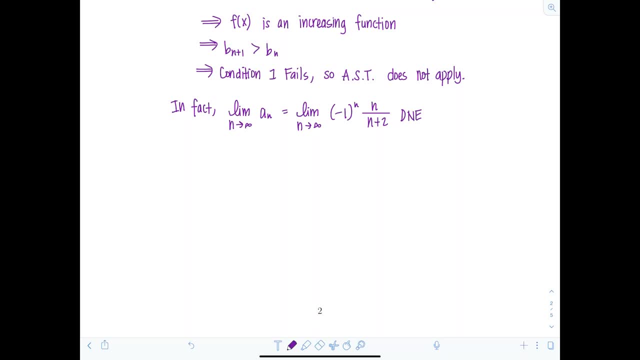 and the odd terms approaching another value. So I'm going to go into a little more detail than probably what's necessary for you, just to demonstrate for this first example, And then from here on out I'll just kind of cut to the chase when we're working these examples. 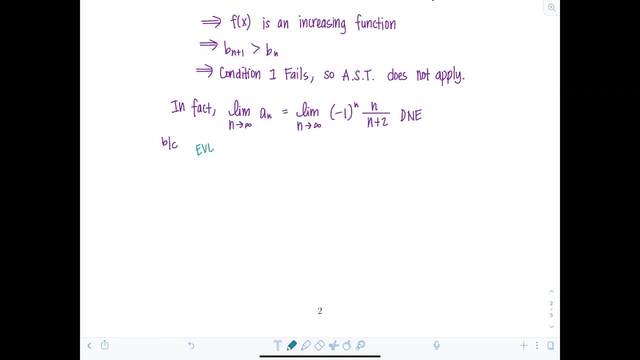 So here's why. So consider the even terms- okay, Those I'm going to look at the limit as n approaches infinity, of all of the even terms of our sequence, a sub n. So those would all be the ones with index 2n, right? 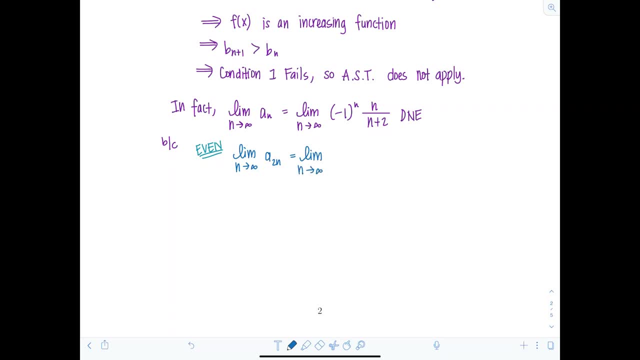 So this would be the limit, as n approaches infinity, of negative 1 to the 2n times 2n over 2n plus 2.. But negative 1 to the 2n, that's going to be negative 1 raised to an even power. 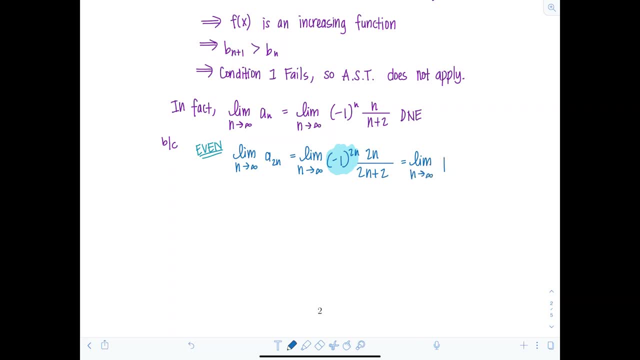 So it's just going to turn into positive 1 times 2n over 2n plus 2.. And then now, when we take this limit, since the degree of the numerator is equal to the degree of the denominator, I can just take the ratio of the leading coefficients. 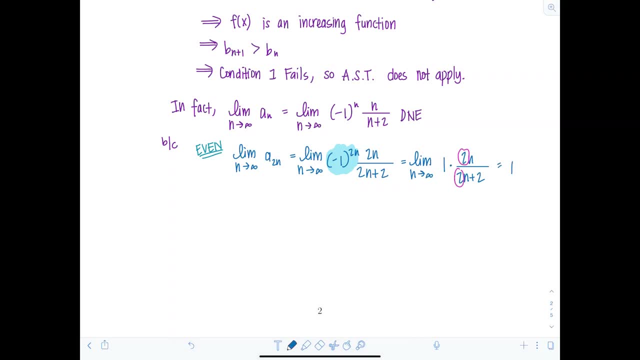 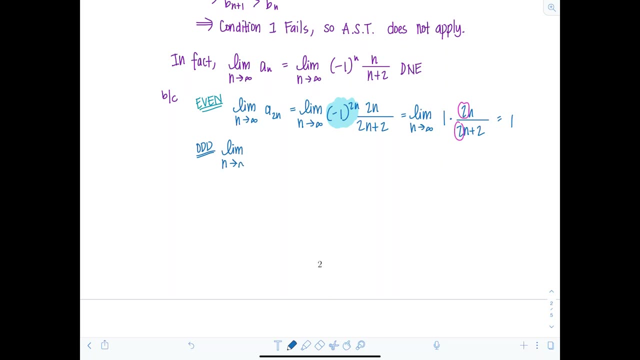 And this limit comes out to be positive: 1.. However, look at the odd terms. So the odd terms, I'm going to look at the limit. as n approaches infinity, The odd terms would be the ones whose index, you know, is negative. 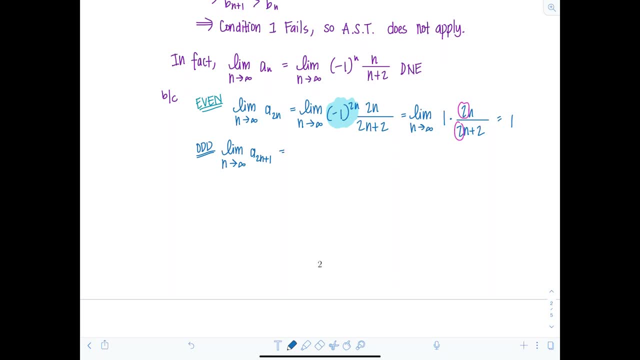 So the odd terms I'm going to look at the limit as n approaches infinity. The odd terms would be the ones whose index, you know, is negative. This 0 is 2n plus 1.. So that would be the limit as n approaches infinity. 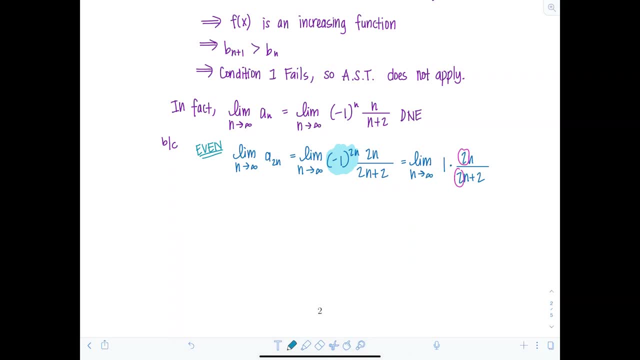 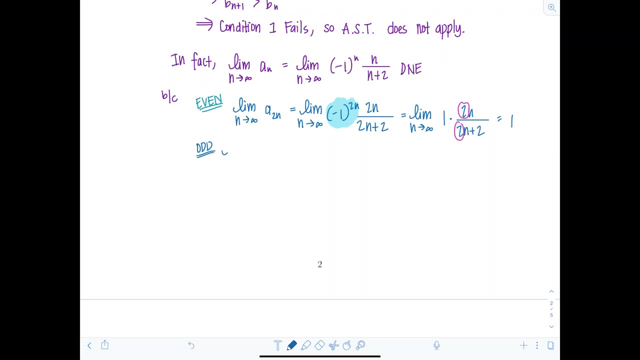 the ratio of the leading coefficients and this limit comes out to be positive 1.. However, look at the odd terms. So the odd terms. I'm going to look at the limit as n approaches infinity. The odd terms would be the ones whose index is 2n plus 1.. So that would be the limit as n approaches. 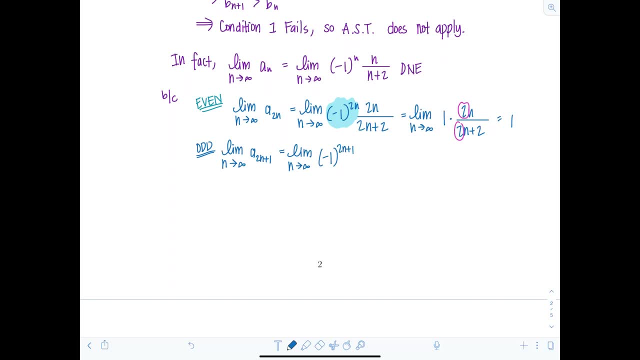 infinity of negative 1 to the 2n plus 1 times 2n plus 1 over 2n plus 3.. And then from here I can look at the limit now as n approaches infinity. Well, be careful, This time negative. 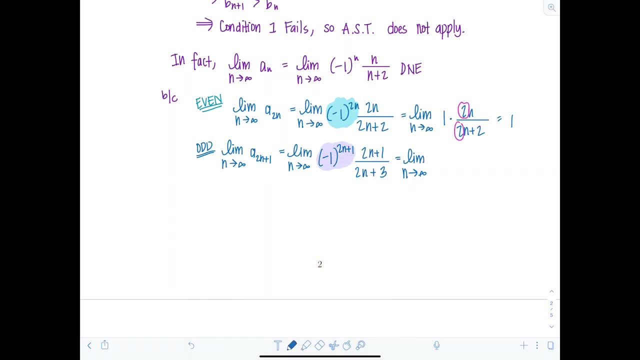 1 is raised to the 2n plus 1, which is an odd number, so that negative is going to remain. So I have negative 1 times 2n plus 1 over 2n plus 3.. Again, degree of the numerator equals the degree of the. 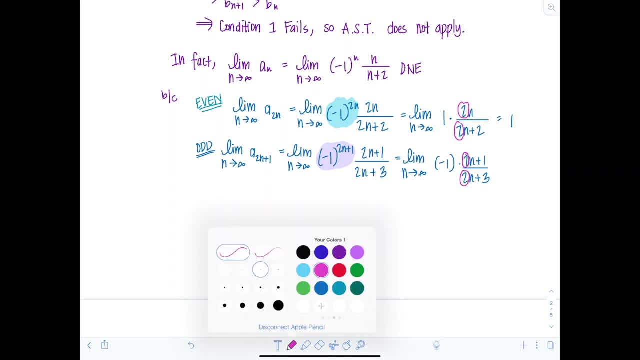 denominator. so I could take the ratio of the leading coefficients. That's going to be 1, but then I still have that negative 1 in the front. So we notice here, because the even terms of the sequence a- n have the limit 1, as n goes to infinity, but the odd terms have a limit of. 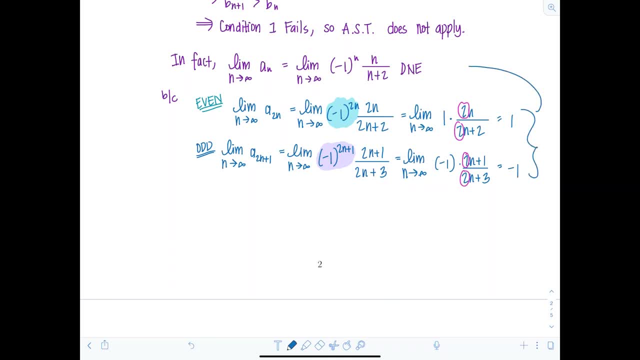 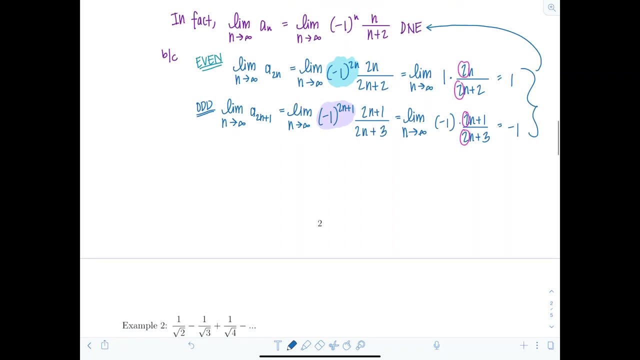 negative 1.. This means that my original sequence does not have a limit. It does not exist. So thus we can say that the limit as n approaches infinity of negative 1 to the n times n over n plus 2, does not exist. and if it does not exist, therefore, it doesn't equal 0. So 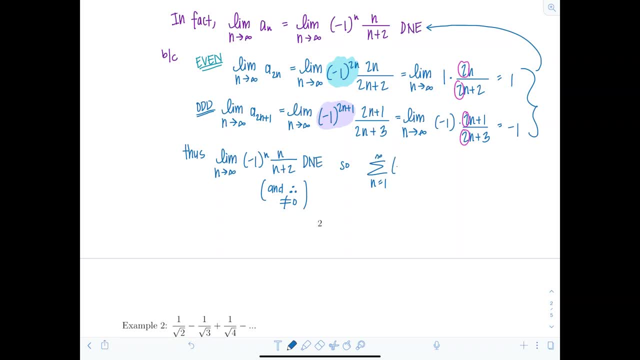 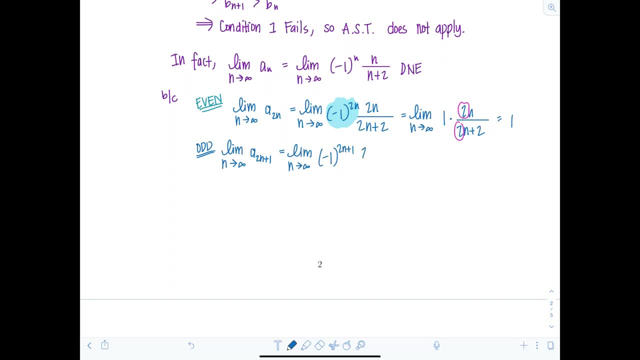 of negative 1 to the 2n plus 1, times 2n plus 1, over 2n plus 3.. And then from here I can look at the limit now as n approaches infinity. We'll be careful this time. 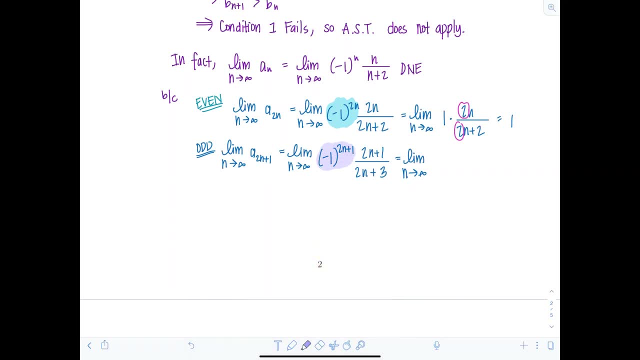 negative. 1 is red raised to the 2n plus 1, which is an odd number, So that negative is going to remain. So I have negative 1 times 2n plus 1 over 2n plus 3.. Again, degree of the numerator equals the degree of the. 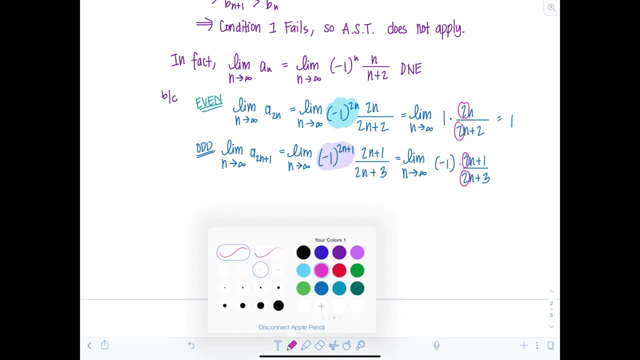 denominator. So I could take the ratio of the leading coefficients. That's going to be 1.. But then I still have that negative 1 in the front. So we notice here, because the even terms of the sequence a- n have the limit 1, as n goes to infinity, but the odd terms have a limit of. 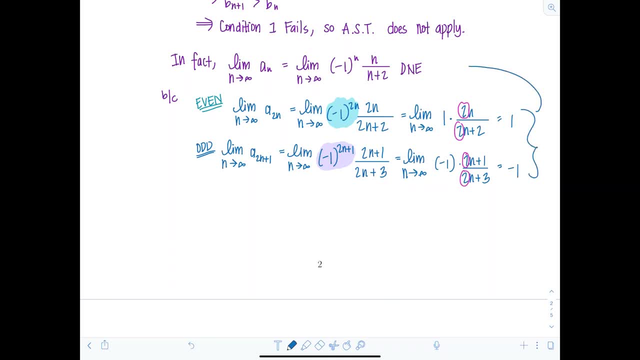 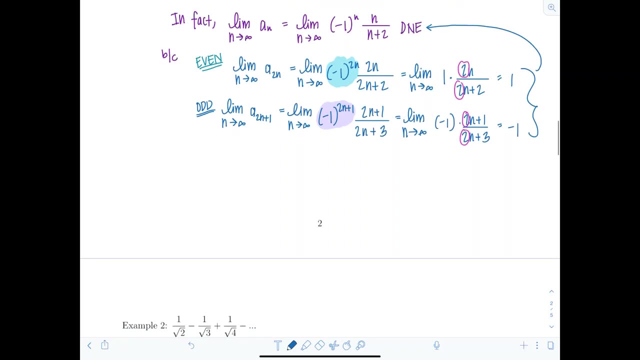 negative 1, this means that my original sequence does not have a limit. It does not exist. So thus we can say that the limit, as n approaches infinity of negative 1 to the n times n over n plus 2, does not exist. And if it does not exist, 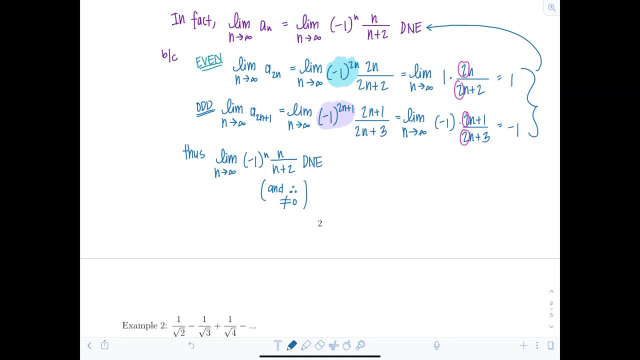 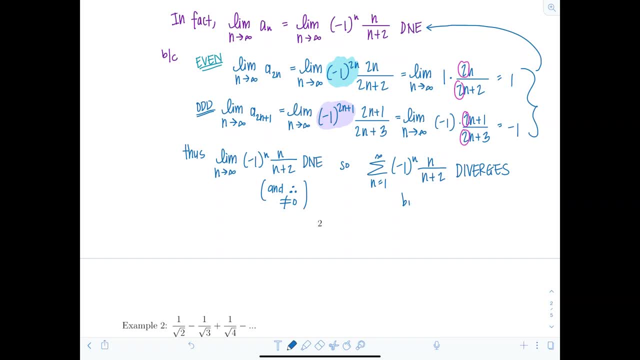 by the test for divergence. Okay, very nice. Now, as far as what's required, you can just list out the conclusion here: Your n equals 1 to infinity of negative, 1 to the n times n over n plus 2. diverges by the test for: 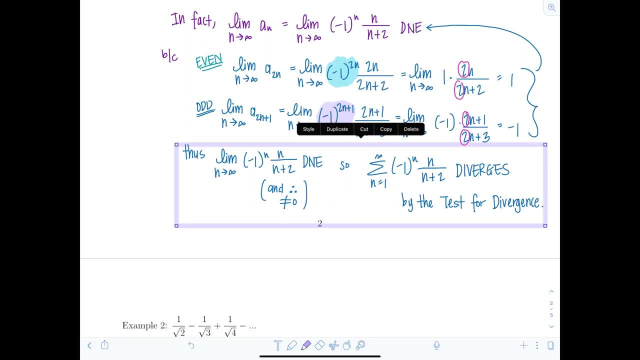 original series. It diverges by the test for divergence and you don't have to go so rigorously into showing the limit of the even and odd terms, as long as you just identify that they go to different places and therefore the limit doesn't exist. That's sufficient for this. 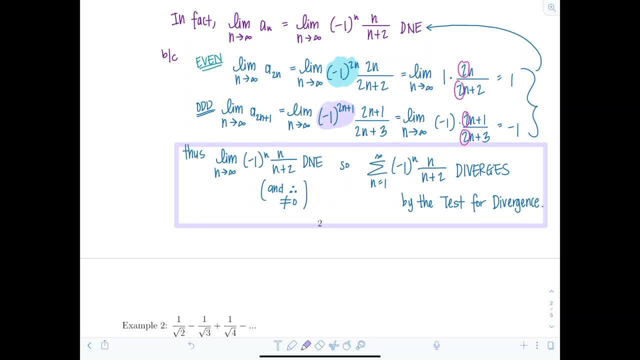 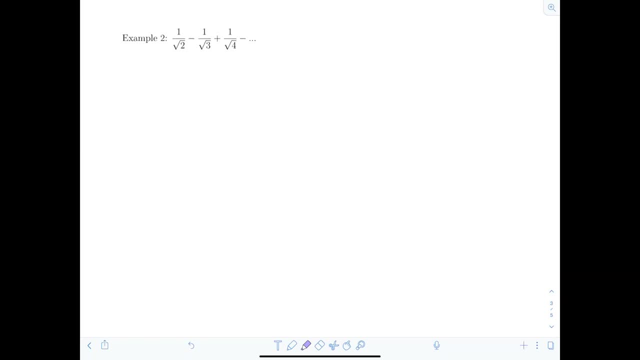 class. Okay, let's move on to another example, Example 2,. we have the following series: 1 over rad 2 minus 1 over rad 3 plus 1 over rad 4, so on and so forth. So let's see here. First let's write. 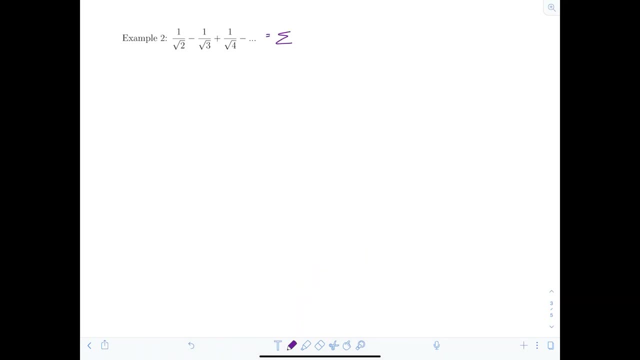 it in sigma notation. So this is going to be the sum n equals. let's just start at 1 to infinity, and I'm going to have 1 over. well, the first denominator needs to have a rad 2, so I'm going. 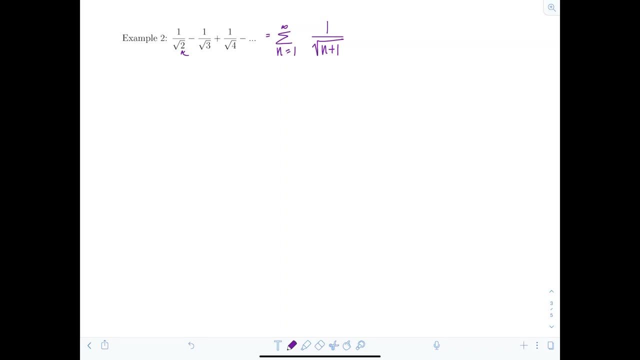 to have rad n plus 1, and then notice my first term is positive, right? So in this case I need negative 1 raised to the n minus 1, not the nth power, because I want that first term to be positive, second one to be negative, etc. 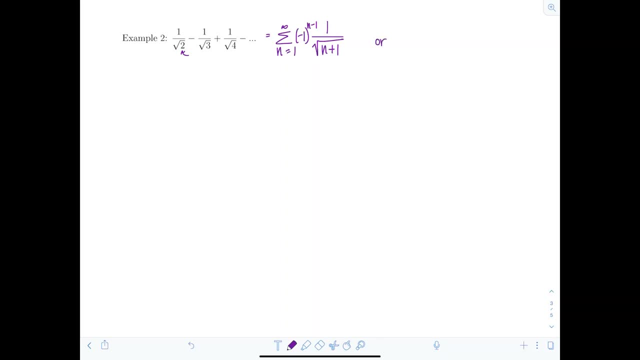 Okay, that's one way to do it. or maybe you're more inclined to start your index at 2, because you notice you had a rad 2 in the denominator. Well then, you would have negative 1 to the n right, Because your first term would be negative 1 squared times 1 over. 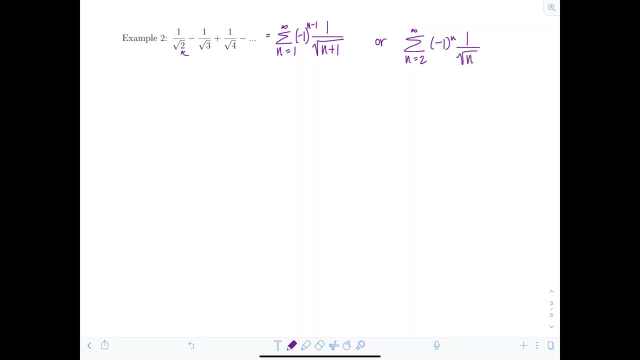 and then now I'm just going to start at rad n. Both are correct. Both will yield the same conclusion. okay, Let's list out, identify what b sub n is. I'm just going to work with the first one. So b sub n is 1 over rad n plus 1.. So I'm going to apply the alternating. 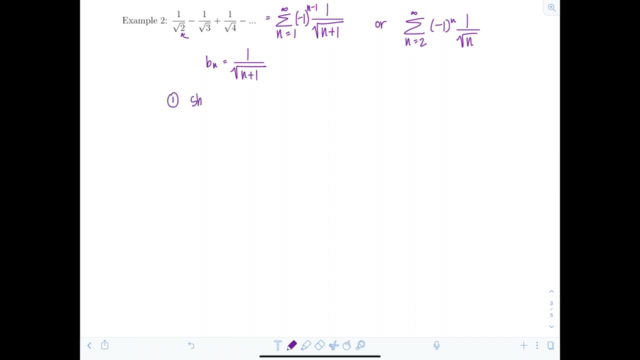 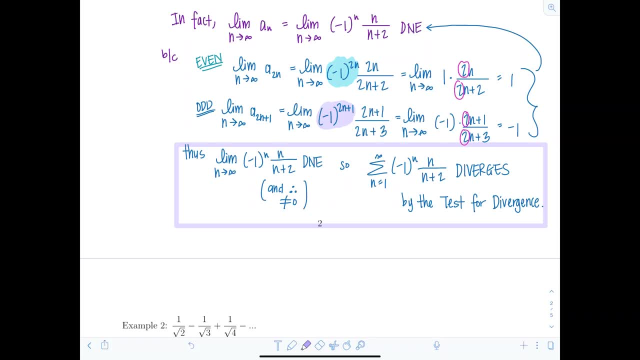 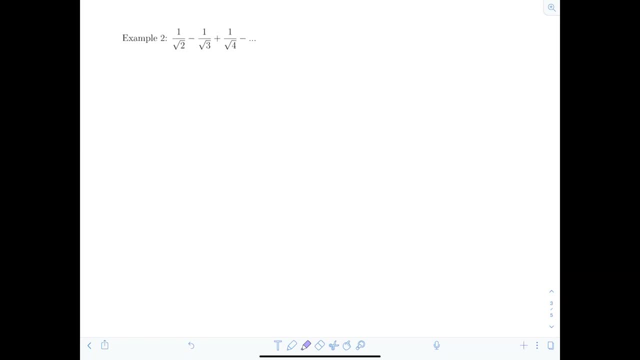 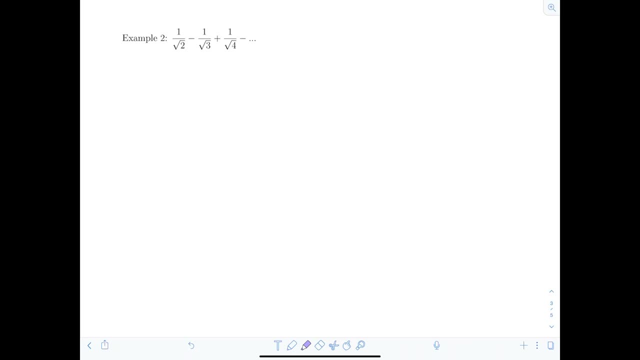 minus 1 over rad 3, plus 1 over rad 4, so on and so forth. So let's see here. First let's write it in sigma notation. So this is going to be the sum n equals. let's just start. 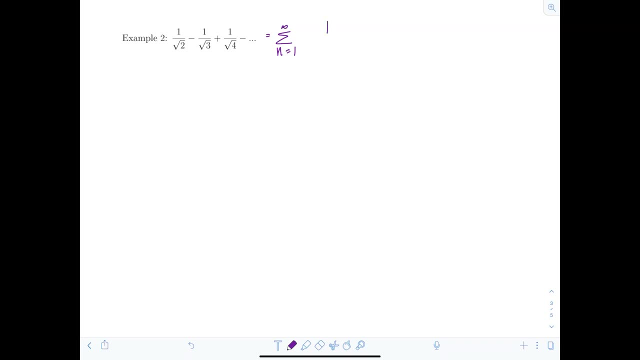 at 1 to infinity, and I'm going to have 1 over. well, the first denominator needs to have a rad 2, so I'm going to have rad n plus 1.. And then, notice, my first term is positive, right, So in: 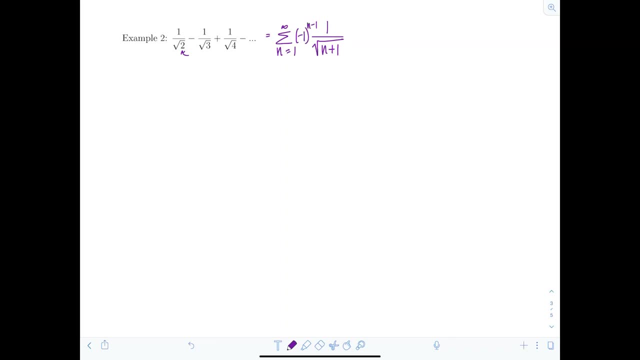 this case, I need negative 1 raised to the n minus 1, not the nth power, because I want that first term to be positive, second one to be negative, etc. Okay, that's one way to do it, or maybe? 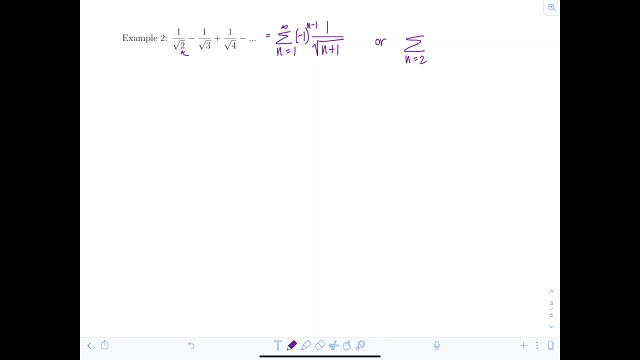 you're more inclined to start your index at 2, because you notice you had a rad 2 in the denominator. Well then you would have negative 1 to the n, minus 1 over rad 2, minus 1 over rad 3. 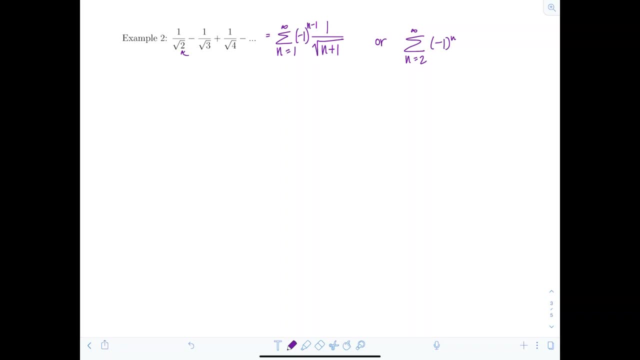 to the n right, Because your first term would be negative 1 squared times 1 over. and then now I'm just going to start at rad n. Both are correct. Both will yield the same conclusion. okay, Let's list out, identify what b sub n is. I'm just going to work with the first one. So b sub n is 1 over. 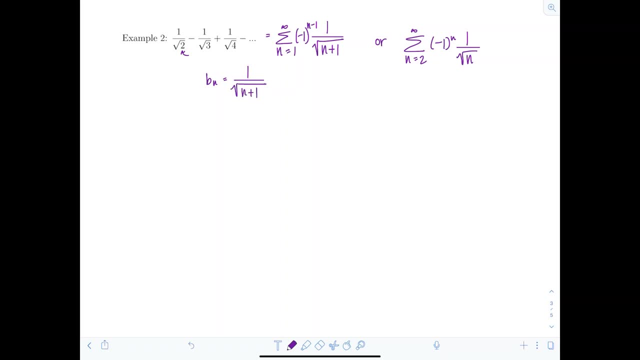 rad n plus 1.. So I'm going to apply the alternating series test. First condition: I know that b sub n plus 1 is less than or equal to b sub n. Well, b sub n plus 1 is 1 over rad n plus. 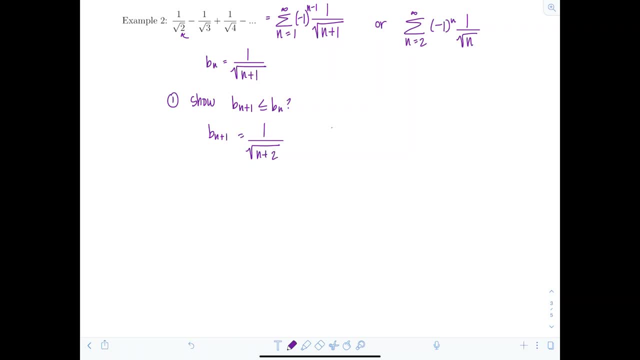 2. And b sub n is just 1 over rad n plus 1.. Well, clearly, I know b sub n plus 1 is smaller, since the denominator is larger, and that's the only part of the expression that changed. 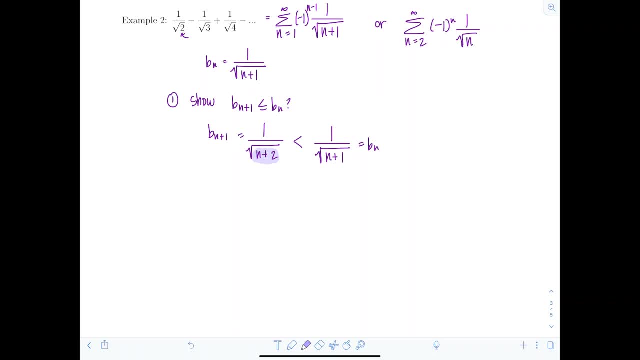 It wasn't like the previous example where both the numerator and denominator were changing in ways that wasn't making the inequality conclusive. So we satisfied the first condition: it's decreasing. And then condition two: I need to show that the limit as n approaches infinity. 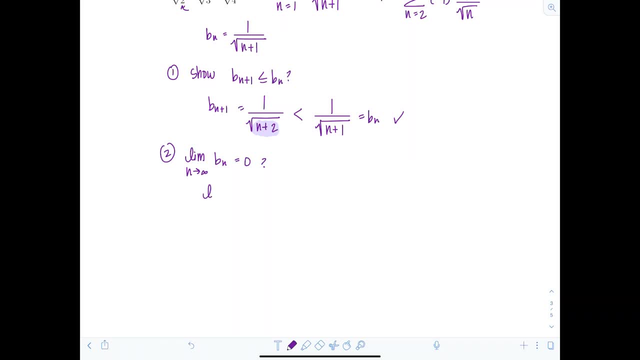 of b sub n is 0.. Can I show that? Well, let's take the limit, as n approaches infinity, of 1 over rad n plus 1.. Well, as n approaches infinity, this denominator is going to get large without bound, approach infinity. So indeed, 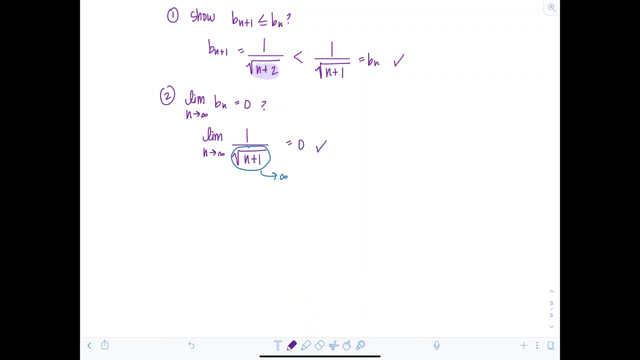 this limit is 0.. Yay, So this implies that our original series- let's write it how it was- 1 over rad 2 minus 1 over rad 3 plus 1 over rad 4 minus dot, dot dot that converges. 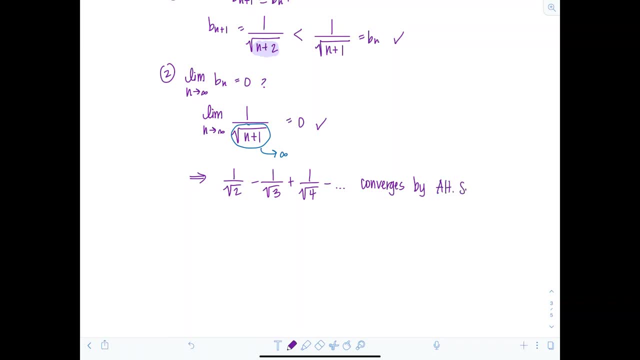 by always state what test you used. alternating series test Beautiful. Okay, looks nice. Let's look at some other examples to see what we could run into. So example three: we have the sum n equals 1 to infinity of negative 1 to. 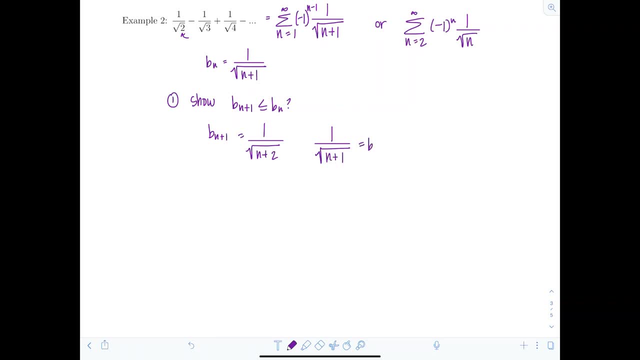 rad n plus 1.. Well, clearly, I know b sub n plus 1 is smaller, since the denominator is larger, and that's the only part of the expression that changed. It wasn't like the previous example where both the numerator and denominator were changing in ways that wasn't making 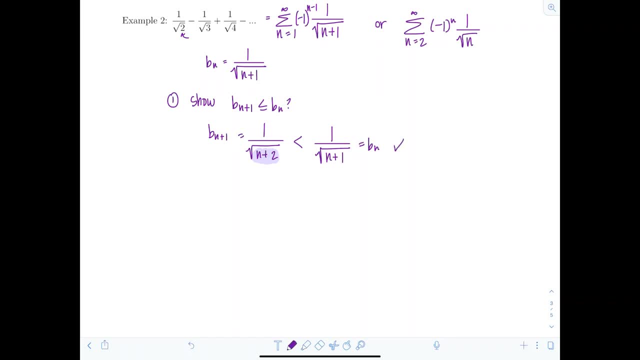 it, the inequality conclusive. So we satisfied the first condition: it's decreasing. And then condition 2, I need to show that the limit as n approaches infinity of b sub n is zero. Can I show that? Well, let's take the limit as n approaches infinity of one. 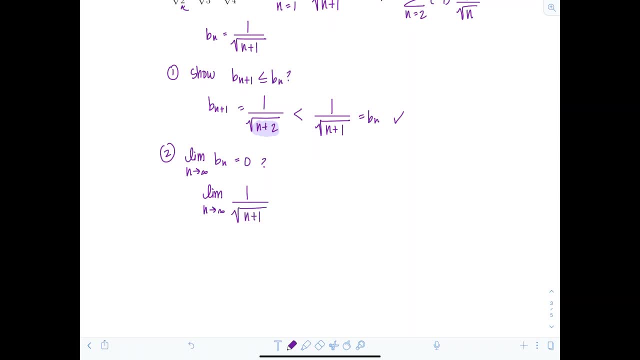 over rad n plus one. Well, as n approaches infinity, this denominator is going to get large without bound. approach infinity. So indeed, this limit is zero. Yay, So this implies that our original series- let's write it how it was- one over rad two minus one over rad three plus one. 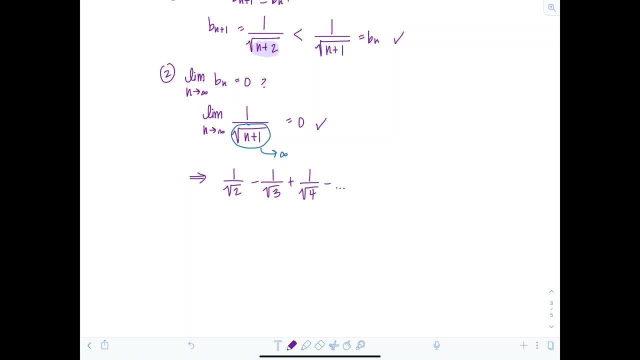 over rad four minus dot dot dot That converges by always state what test you used, the alternating series test Beautiful, Okay, Looks nice. Let's look at some other examples to see what we could run into. So example three: we have the sum n equals one to infinity, of negative one to the n times n. 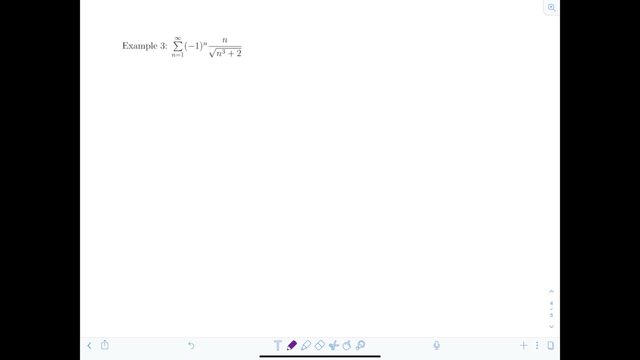 over the square root of n cubed plus two. Okay, So I'm going to list off to the side here. b sub n is n over the square root of n cubed plus two. So first I want to show you that I have a square root of n cubed plus two. 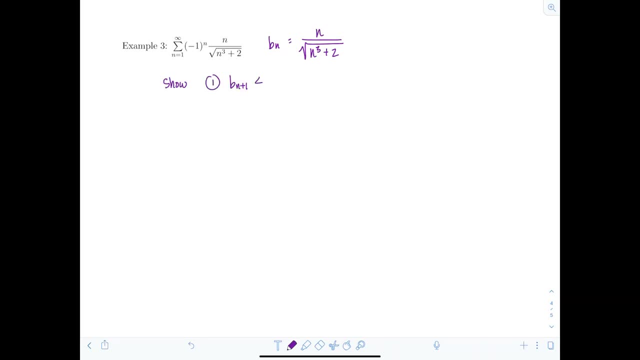 Now let's see. can I show that b sub n plus one is less than or equal to b sub n? Well, let's see: b sub n plus one, that would be n plus one over the square root of n plus one cubed plus two. And b sub n is just n over rad n cubed plus two. 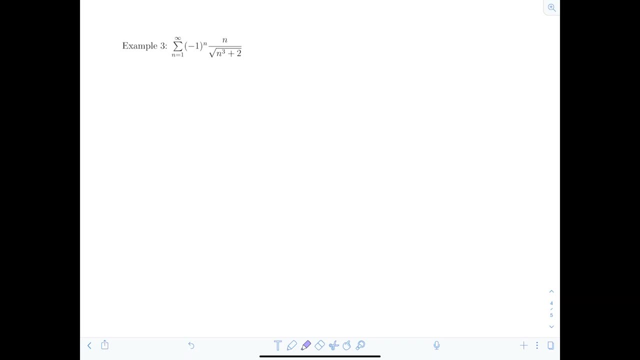 the n times n over the square root of n cubed plus 2.. Okay, so I'm going to list off to the side here. b sub n is n over the square root of n cubed plus 2.. So first I want to see: can I show that b sub n plus 1 is less than or equal to b sub n? 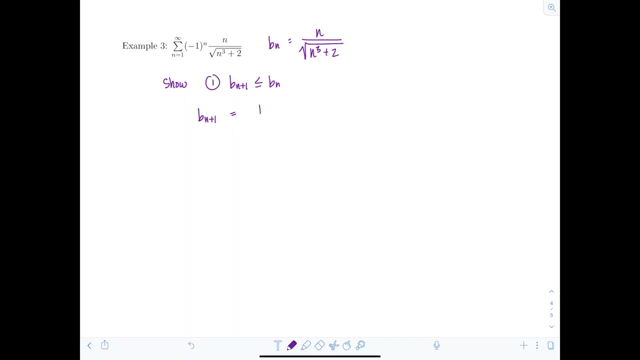 Well, let's see b sub n plus 1, that would be n plus 1 over the square root of n plus 1 cubed plus 2.. And b sub n is just n over rad n, cubed plus 2.. Can I show a clear inequality in one direction or? 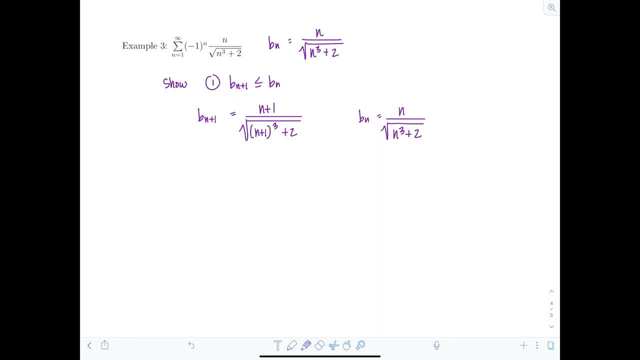 another. Well, in this case no, because the denominator increased, yes, but then so did the numerator. So who's to say? It's not obvious? So in that case it's time to take the derivative. So first we're going to define our function. let f of x equal. 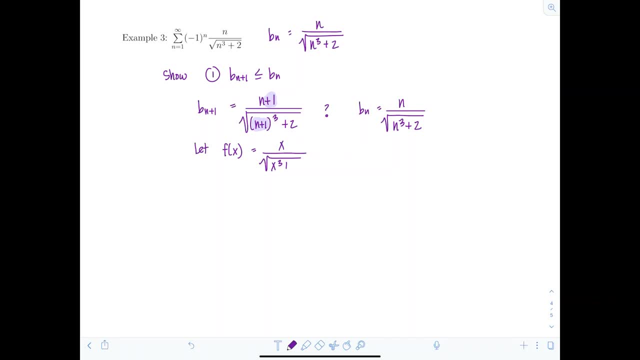 x over rad x cubed plus 2.. And then it's derivative time, So let's go ahead, apply the quotient rule here. So f prime of x is going to be rad x cubed plus 2 times derivative of the numerator, which is just 1,. 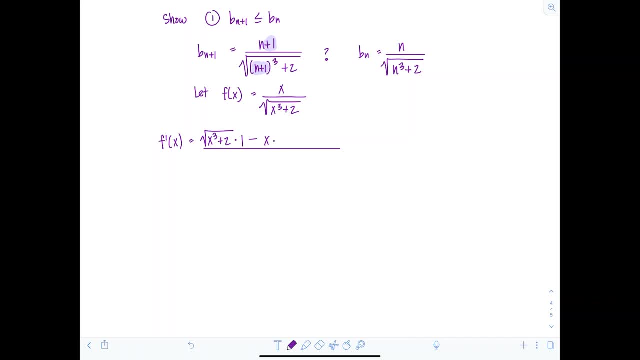 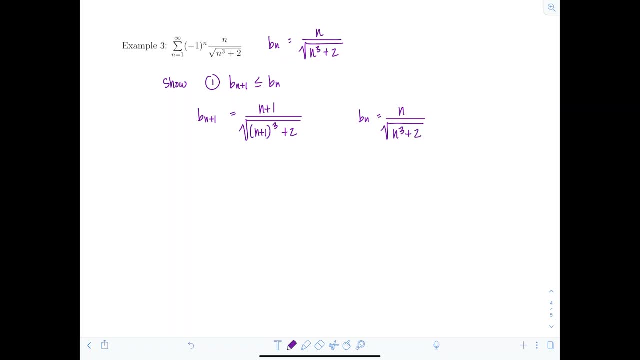 Can I show a clear inequality in one direction another? Well, in this case no, because the denominator increased, yes, but then so did the numerator. So who's to say It's not obvious? So in that case, it's time to take the derivative. 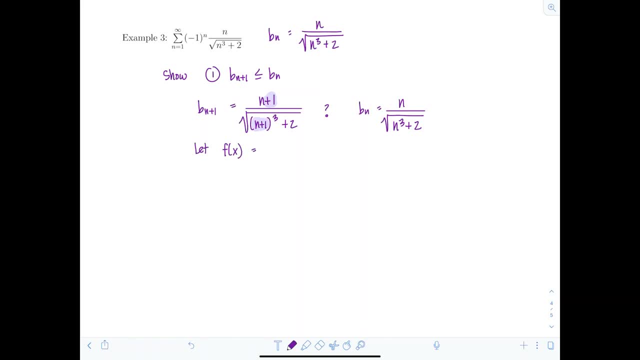 So first we're going to define our function. Let f of x equal x over rad x cubed plus 2.. And then it's derivative time, So let's go ahead, apply the quotient rule here. So f prime of x is going to be: 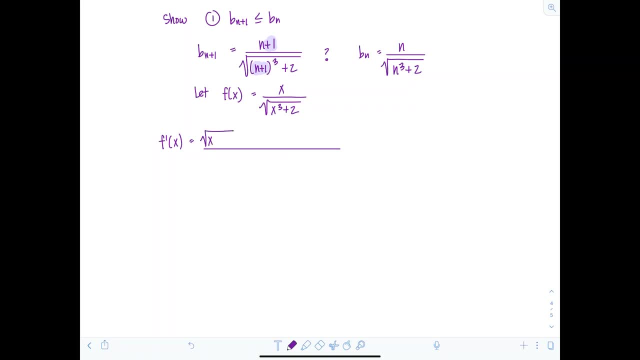 rad x cubed plus 2 times derivative of the numerator, which is just 1, minus. I have the numerator x times derivative of the denominator. So that's rad x cubed plus 2, or x cubed plus 2 to the 1 half power. So I'm going to have 1 half x cubed plus 2 to the negative. 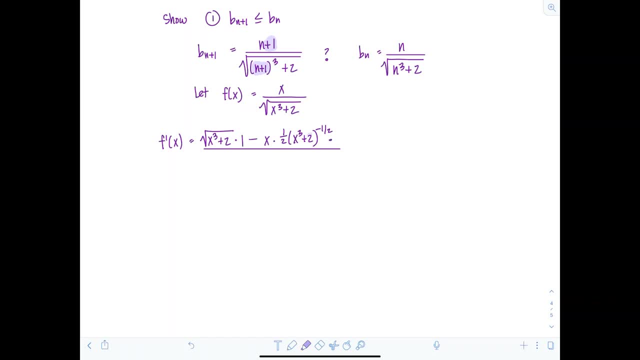 1 half times by the chain rule derivative of the infinite Derivative of x cubed plus 2, which is 3x squared. And then all this goes over the denominator squared, which is just going to be x cubed plus 2, no more radical. 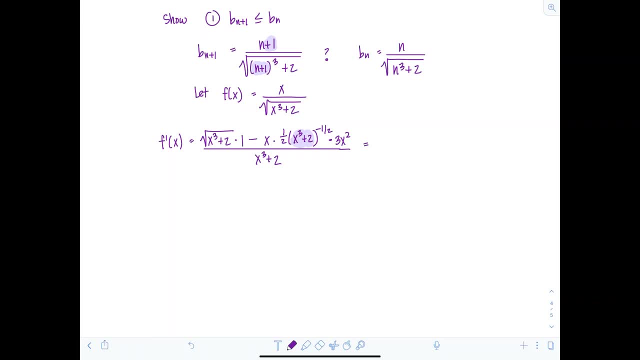 Okay, let's clean things up a bit here. So we have rad x cubed plus 2 minus. now notice I have this negative exponent And then I want to. I want to list that quantity in the denominator so I can see how to completely simplify or clean. 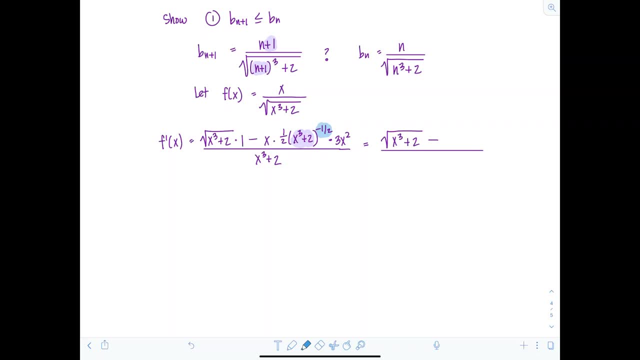 up this derivative. I can put the 3 over the 2, and then I'm going to have an x cubed in the numerator. So this is going to become 3x cubed over 2 times rad, x cubed plus 2.. And then I have 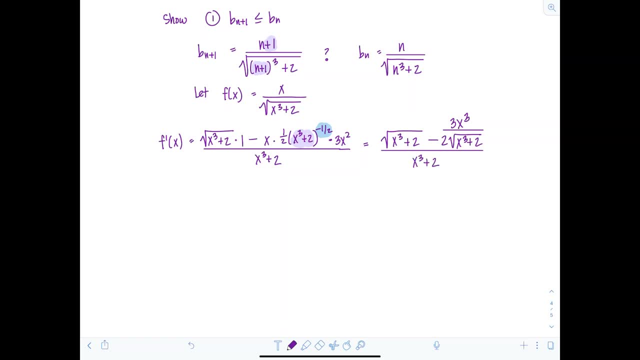 x cubed plus 2 hanging out down there in the denominator. Okay, so this is a complex fraction, right? We can't have a fraction within a fraction And I need- I need to simplify because I have to figure out if it's positive or negative. And right now, when. 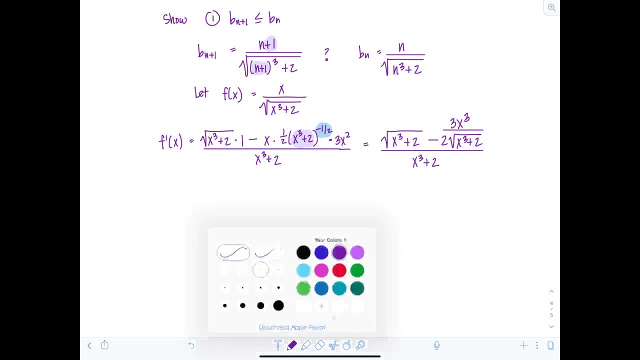 it's all messy, it's of no use to me. So I want to multiply through by the LCD to clear out those denominators, that extra denominator. So I'm going to multiply by 2, rad x, cubed plus 2. And then I 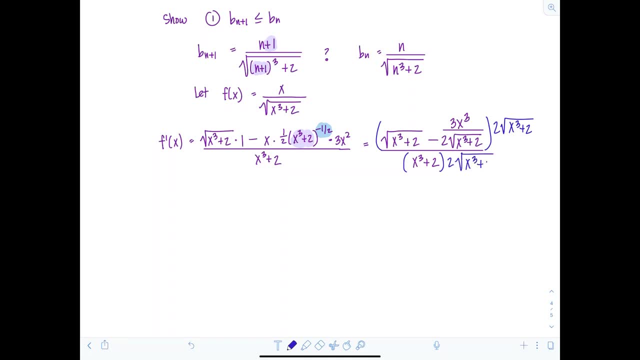 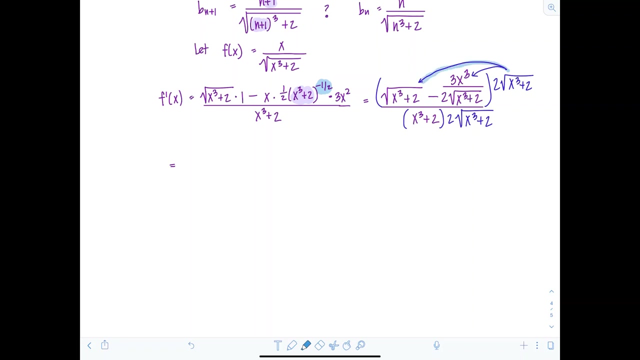 need to multiply by the same thing in the denominator 2: rad x cubed plus 2.. And we will distribute here. Okay, now let's see. Notice: the nice thing is, when I distribute I'm going to distribute across to the first term here. The rad x cubed plus 2 times rad x cubed plus 2 is just. 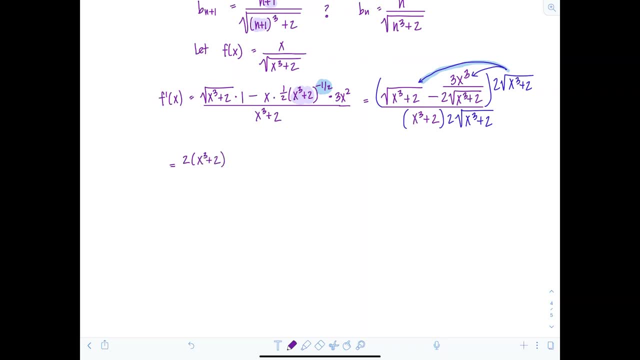 going to give me an x cubed plus 2.. So I have 2 times x cubed plus 2, minus, and then now this whole denominator is gone. Yay, So minus 3x cubed over 2, put the 2 out in the front, And then you: 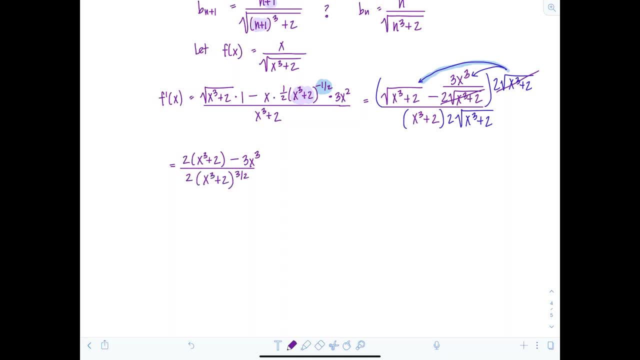 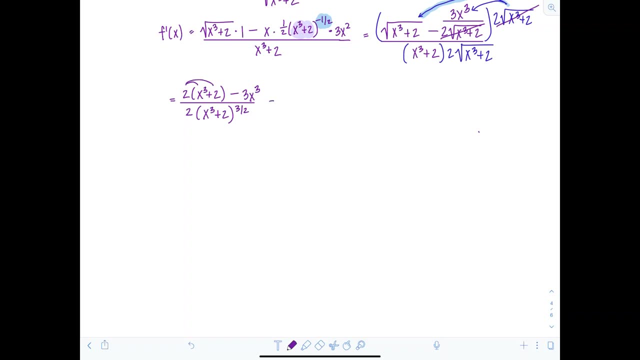 just have x cubed plus 2 to the 3 halves tower. All right, looks good. Looks good. Then from here we can distribute and simplify the numerator, So we'll end up with a negative x cubed plus 4 over 2 times x cubed plus 2 to the 3 halves. 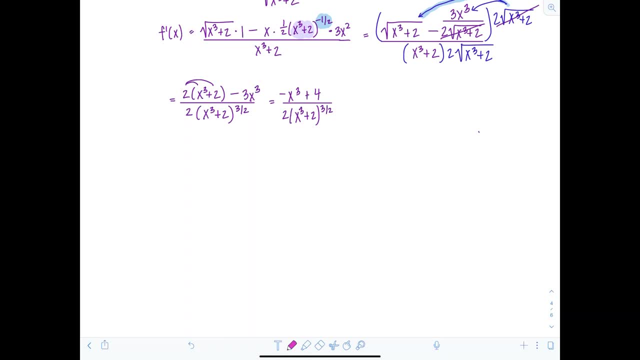 Okay, so what can we say about this derivative? Well, looking at the denominator, it's always going to be positive, right? If I something to the 3 halves power, it's not going to turn out to be negative. And then the numerator negative: x cubed plus 4.. As long as x is larger than the cube root of 4,. 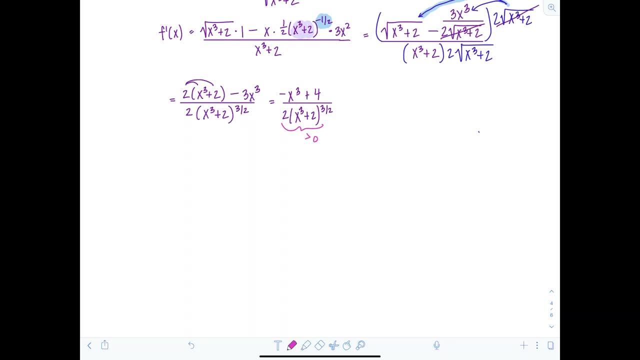 which is a little more than 1 and a half. then the numerator is going to be negative, So I can say that this derivative is going to be less than 0. It's going to be negative for all x's that are greater than or equal to 2, being safe. And I can say this because 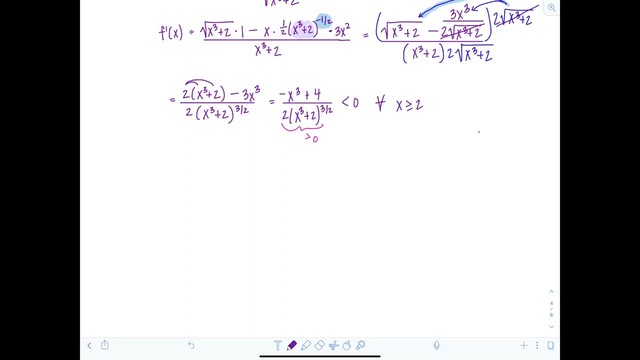 remember I'm going to be negative. I'm going to be negative for all x's that are greater than or equal to 2.. So I'm really interested in if bn that sequence- is decreasing. And remember I'm only going to be substituting in natural numbers for n. 1,, 2,, 3, etc. So as long as I 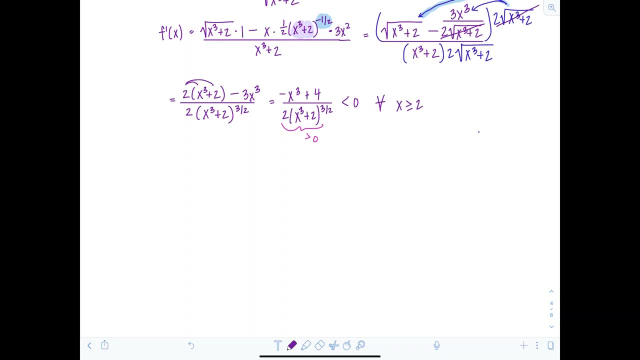 can guarantee x is greater than or equal to 2, then I can say: this function is going to be decreasing, And so the sequence bn is also decreasing eventually, right? So this means it's eventually decreasing, which is good enough for our purposes. 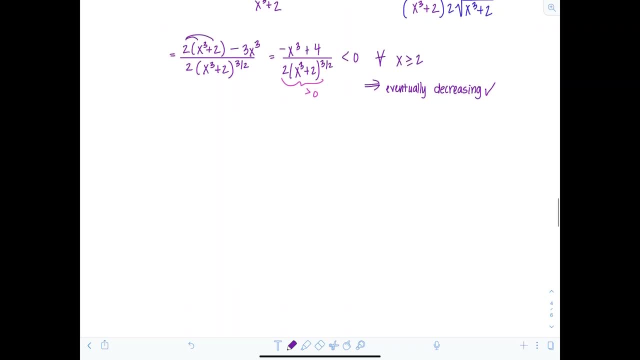 All right, Now I need to check the second condition. Is the limit as n approaches infinity of bn equal to 0?? So let's look at the limit as n approaches infinity of n over the square root of n cubed plus 2.. Now when I take this infinite limit, I want to divide by the highest power of n. 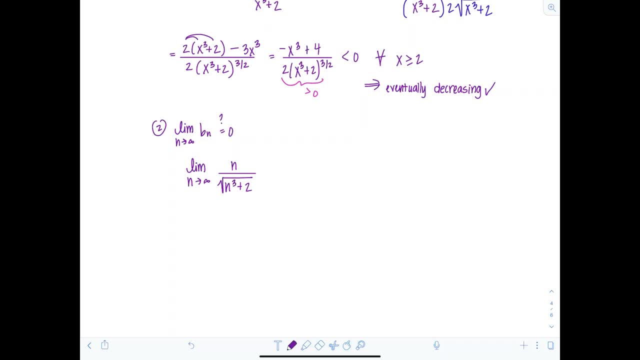 in the denominator, which in this case is n cubed, But remember, since it's underneath the square root, it's really n to the 3.. So I'm going to multiply numerator and denominator by 1 over n to the 3 halves. 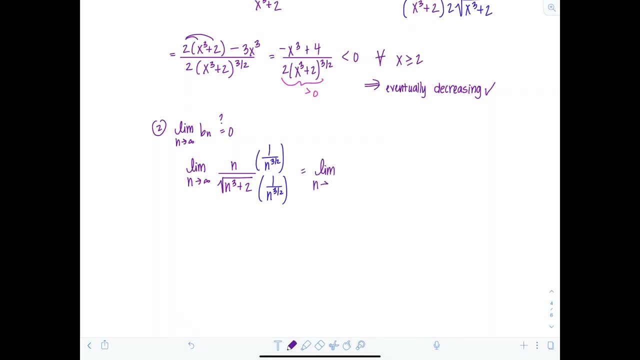 And then distribute that through. So now I have the limit as n approaches infinity And the numerator will have n over n to the 3 halves. So that's 1 over n to the 1 half power. And then in the denominator, when I distribute 1 over n to the 3 halves, underneath the radical. 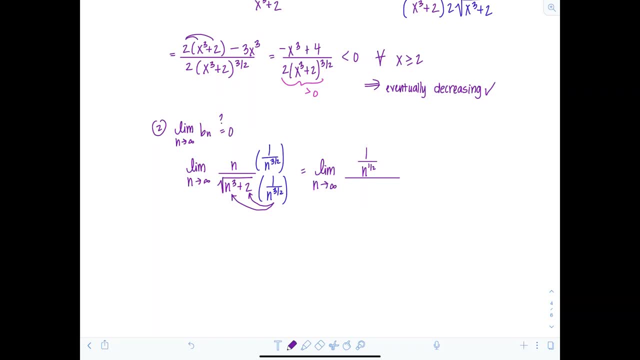 remember I have to square it. So it's going to become 1 over n to the 3 halves 1 over n cubed, And then, multiplying that by n cubed, I'm going to get 1 plus 2 over n cubed. 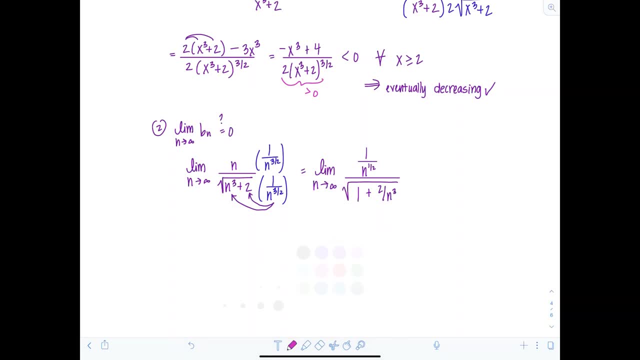 Great, Now as I take the limit. if n goes to infinity, then 1 over n to the 1 half of the numerator will approach 0.. In the denominator underneath the radical 1 is a constant 2 over n cubed that approaches 0. So all I'm going to be left with is 0 over 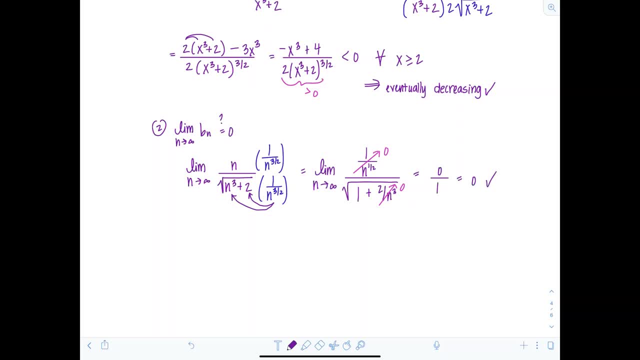 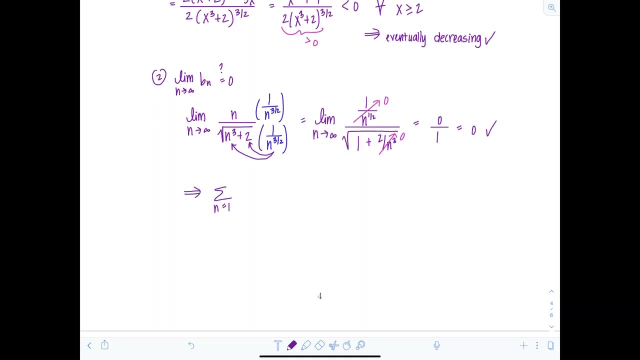 the square root of 1, which is 1, which is 0. So condition 2 is satisfied. This tells me that my original series, the sum n equals 1 to infinity, negative, 1 to the n times n over the square root of n, cubed plus 2, converges. how do I know? By the alternating 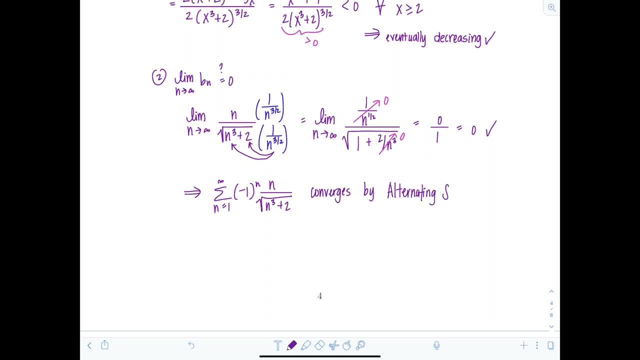 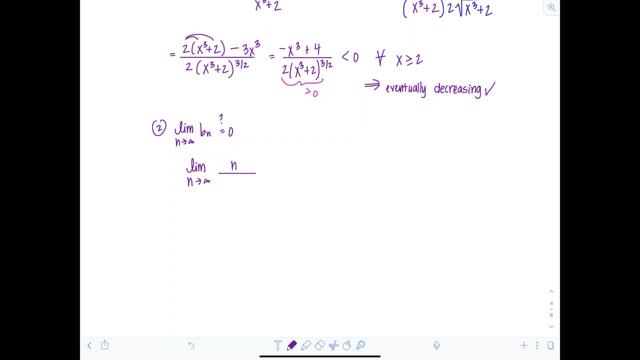 So that's rad x cubed plus 2 to the 1.. So that's rad x cubed plus 2 to the 1. of n over the square root of n, cubed plus 2.. Now, when I take this infinite limit, I want to divide. 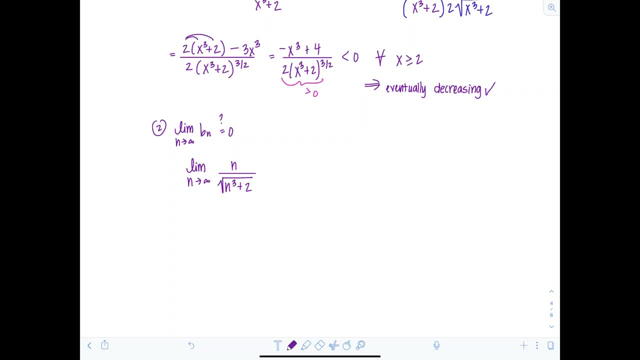 by the highest power of n in the denominator, which in this case is n cubed, But remember, since it's underneath the square root, it's really n to the 3 halves power. So I'm going to multiply numerator and denominator by 1 over n to the 3 halves and then distribute that through. 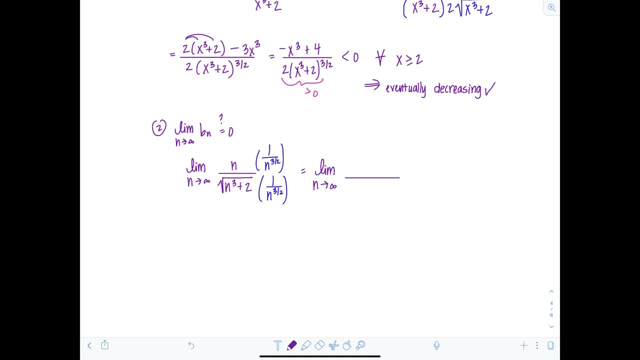 So now I have the limit as n approaches infinity And the numerator will have n over n to the 3 halves, so that's 1 over n to the 1 half power. And then in the denominator, when I distribute 1 over n to the 3 halves underneath the radical, remember I have to square it. so it's going to. 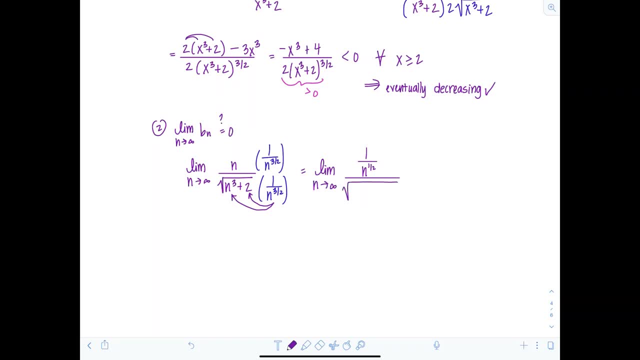 become 1 over n cubed And then, multiplying that by n cubed, I'm going to get 1 plus 2 over n cubed. Great, Now, as I take the limit. if n goes to infinity, then 1 over n to the 1 half of the numerator will. 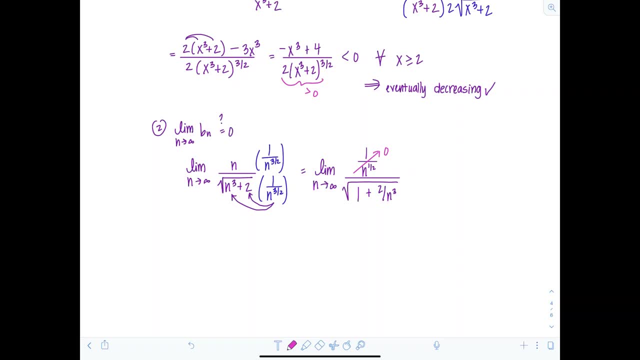 approach 0.. In the denominator underneath the radical 1 is a constant 2 over n cubed that approaches 0. So all I'm going to be left with is 0 over the square root of 1, which is 1,. 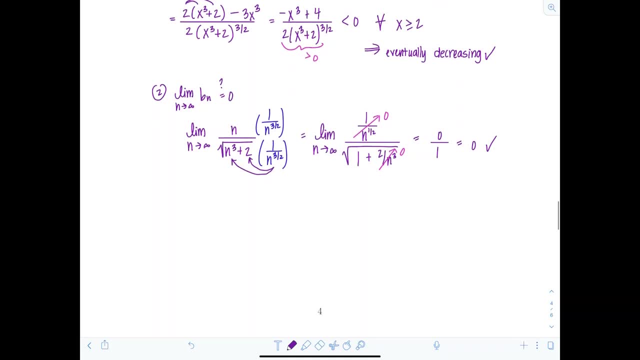 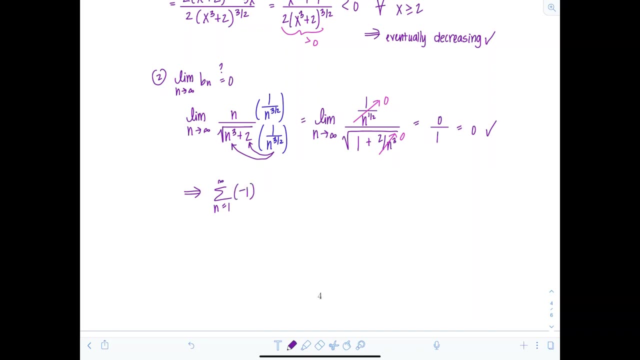 which is 0.. So condition 2 is satisfied. This tells me that my original series, the sum n, equals 1 to infinity, negative 1 to the n times n over the square root of n, cubed plus 2, converges. 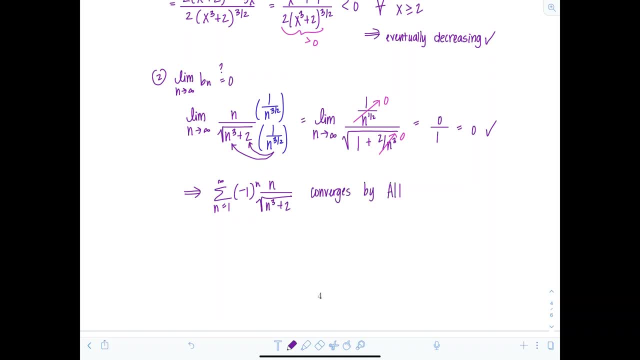 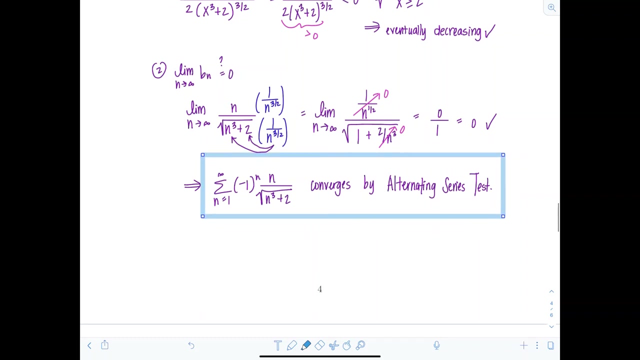 how do I know? By the alternating series test. All right, let's box it. Voila, Example 4, we have the sum n equals 1 to infinity of negative, 1 to the n times 3n raised to the nth power over n factorial. So let's check the first condition. 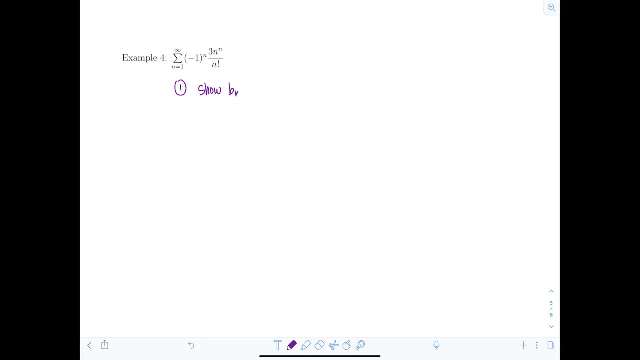 I need to show that b sub n plus 1 is less than or equal to b sub n. Can I do it? Let's identify b sub n. That's going to be 3n to the n Over n factorial. So b sub n plus 1 is going to be 3 times n plus 1. 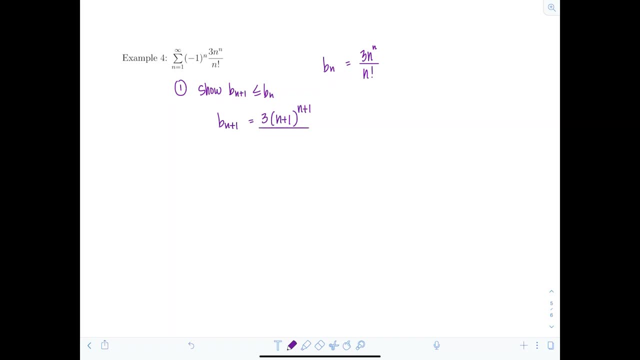 raised to the n plus 1 over n plus 1 factorial And then if I compare that with b sub n, I mean there he was. What can I say? It's not very obvious. The denominator has an extra term. The numerator has also increased. 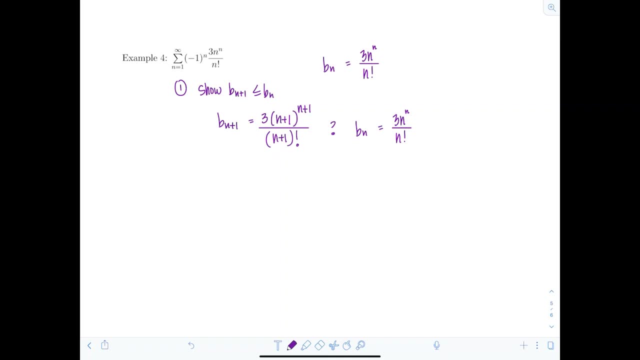 Who's to say? I definitely don't want to take a derivative with a factorial. It's not happening. So let's move on to condition 2.. Maybe that will be more revealing. So, condition 2, let's consider the limit as n approaches infinity, of b sub n. So that's going to be the limit. 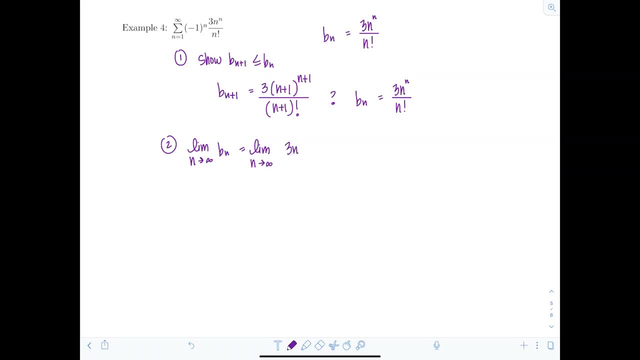 as n approaches infinity of 3n to the nth, Over n factorial. Well, how do you take this limit? I have n raised to the nth power. I have an n factorial. I'm going to rewrite this expression so we can kind of get a better. 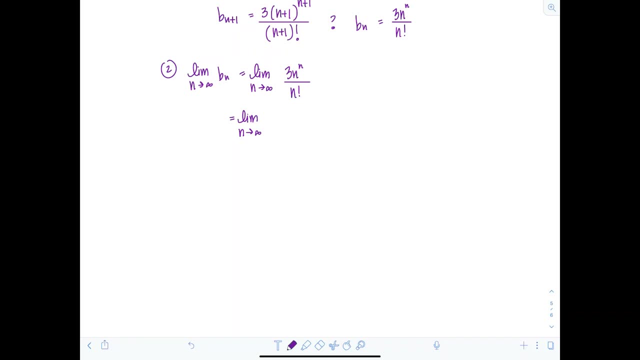 feel for what's going on. Let's just bring that 3 outside And then notice in the numerator I have n raised to the nth power. So that means I have n multiplied by itself, n, many times, right, n times, All right. Now the denominator is n factorial, which you'll remember, that's n times n minus 1. 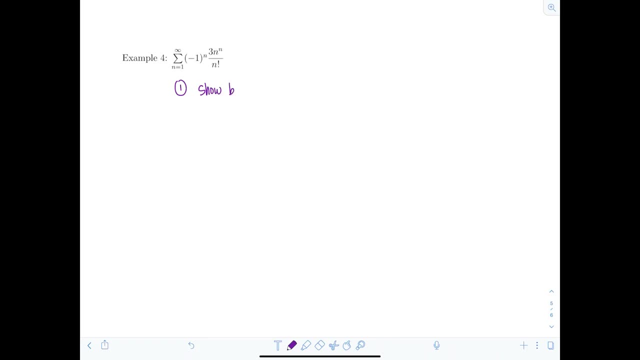 I need to show that b sub n plus 1 is less than or equal to b sub n. Can I do it? Let's identify b sub n. That's going to be 3n to the n over n factorial. So b sub n plus 1 is going to be 3 times n plus 1 raised to the n plus 1 over n plus 1 factorial. 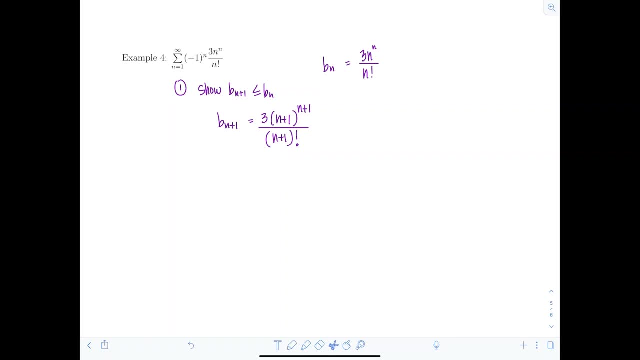 And then if I compare, if I compare that with b sub n- I mean there he was. What can I say? It's not very obvious. The denominator has an extra term. The numerator has also increased. Who's to say? I definitely don't want to take a derivative with a factorial. It's not happening. 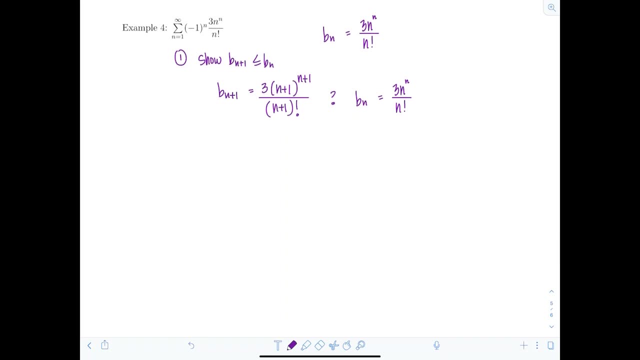 So let's move on to condition 2.. Maybe that will be more revealing. So condition 2, let's consider the limit. So that's going to be the limit as n approaches infinity of b sub n. So that's going to be the limit as n approaches infinity of 3n to the n over n factorial. 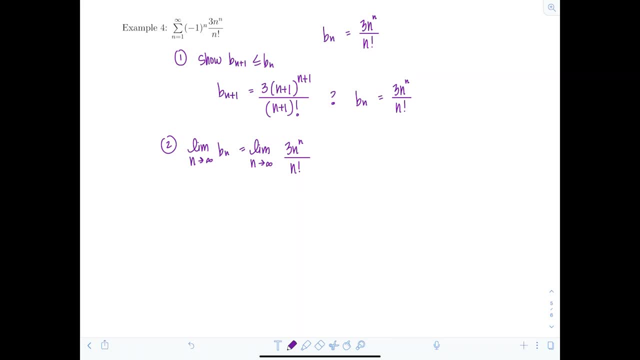 Well, how do you take this limit? I have n raised to the nth power. I have an n factorial. I'm going to rewrite this expression so we can kind of get a better feel for what's going on. Let's just bring that 3 outside And then notice in the numerator: I have n. 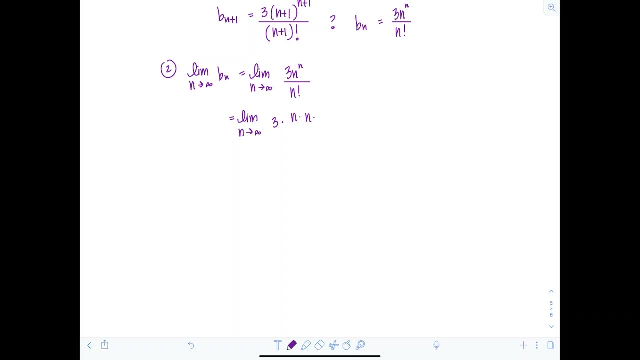 raised to the nth power. So that means I have n multiplied by itself n many times, right n times. All right. Now the denominator is n factorial, which you'll remember, that's n times n minus 1 times n minus 2, all the way down to 1.. Or you could think of it as 1 times 2 times 3. 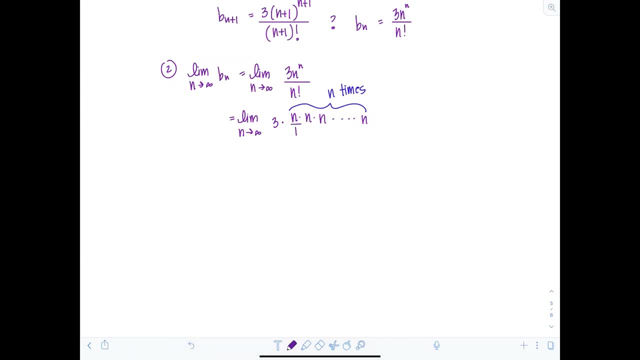 all the way up to n. So that's how I'm going to actually break it down. So it's 1 times 2 times 3, all the way up to n. all right Now. notice each of these terms, except for the last one: n over n. 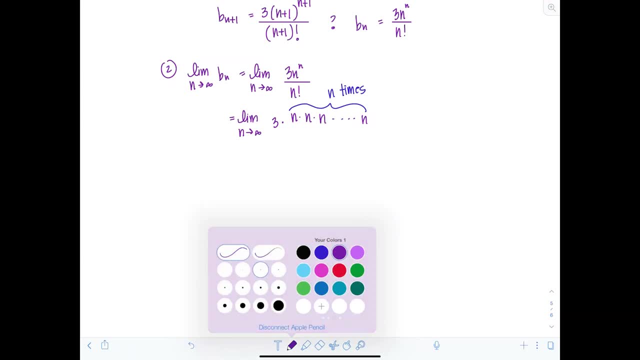 times n minus 2, all the way down to 1.. Or you could think of it as 1 times 2 times 3, all the way up to n. So that's how I'm going to actually break it down. So it's 1 times 2 times 3, all the. 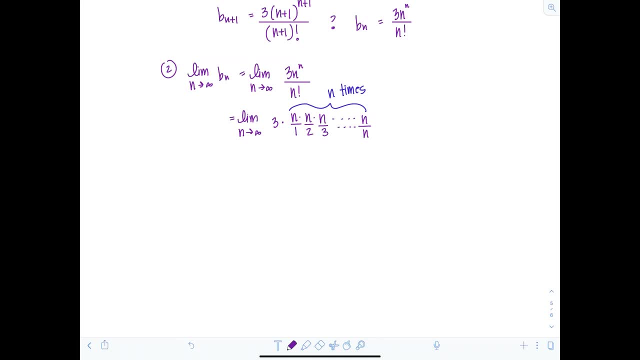 way up to n. All right, Now notice each of these terms, except for the last one: n over n. each of these little factors is greater than 1.. n over n is 1.. And then all of the other terms. the numerator is larger than the denominator, So 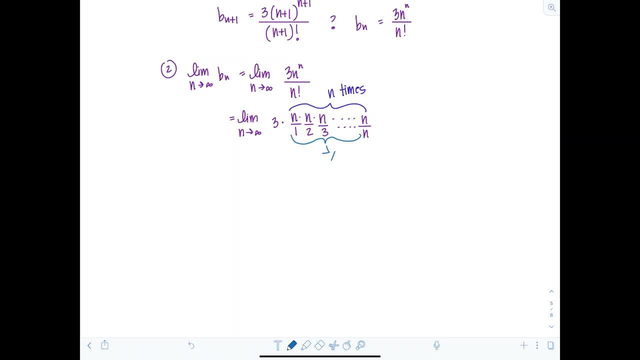 they're greater than 1.. And as n goes and approaches infinity in our limit here, each of those factors is going to get larger and larger, And so this limit ends up approaching infinity, which is definitely not 0.. So condition 2 fails, which means that the alternating series test. 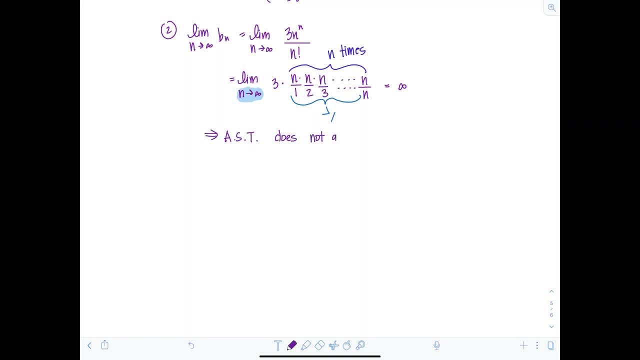 does not apply. And then remember, now, most of the time we can just apply the test for divergence and be done with it. So in fact, the limit as n approaches infinity of a sub n- remember test for divergence if the terms of our original series a, n, do not go to 0,. 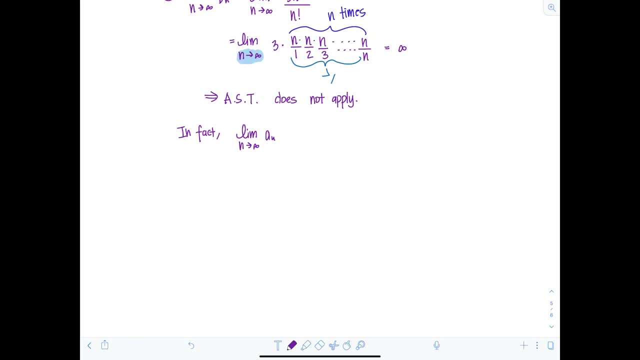 then game over. You can say the series diverges. So I'm looking at the limit as n approaches infinity of a sub n. That's the limit as n approaches infinity. Include the alternating part 3n to the n over n factorial. I know it. 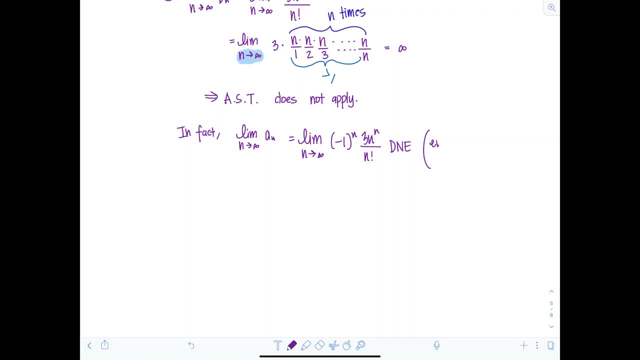 does not exist. Why is that? And all you need to state is that the even terms, they're going to approach infinity And the odd terms they will approach negative infinity, And I'm basing that conclusion on the result from condition 2 failing. 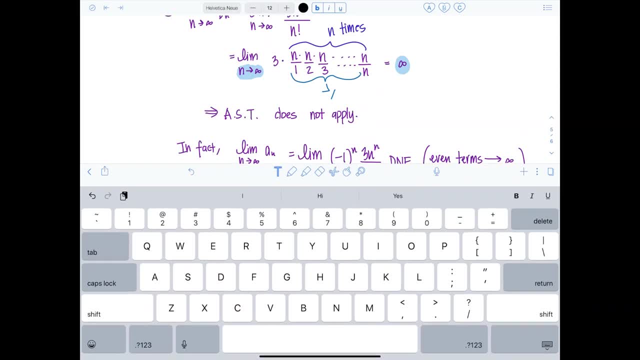 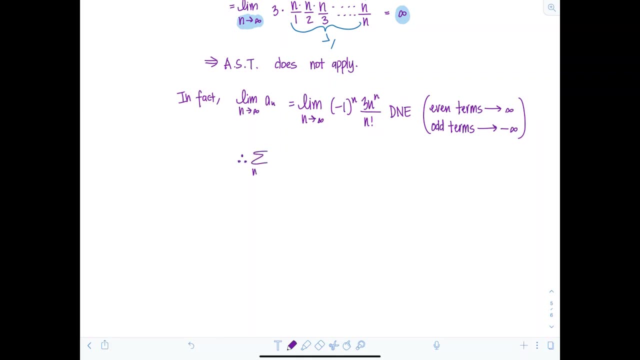 So what is the result? What does this tell me? Ooh Well, therefore, the sum n equals 1 to infinity of negative, 1 to the n times 3n to the n over n factorial diverges by the test for divergence. 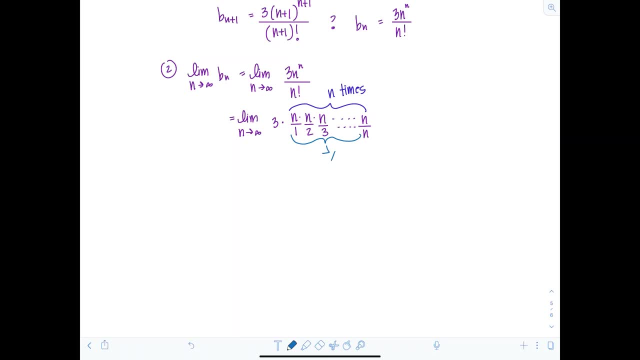 each of these little factors is greater than 1.. n over n is 1, and then all of the other terms. the numerator is larger than the denominator, so they're greater than 1.. And as n goes and approaches infinity in our limit here, each of those factors is going to get larger and larger. 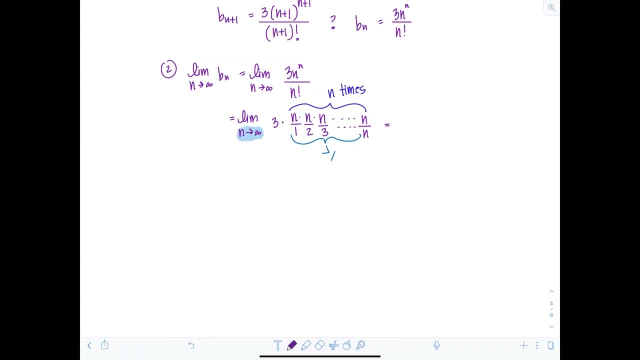 and so this limit ends up approaching infinity, which is definitely not 0. So condition 2 fails, which means that the alternating series test does not apply. And then, remember now, most of the time we can just apply the test for divergence. 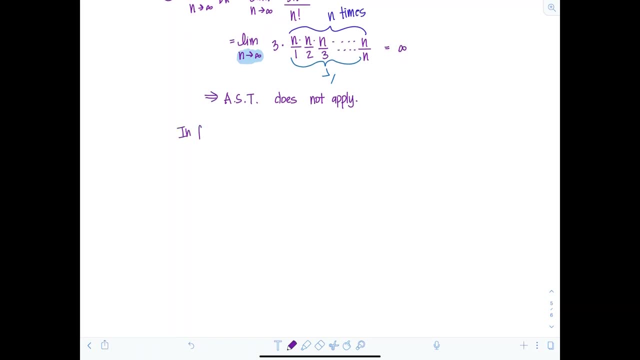 and be done with it. So in fact, the limit as n approaches infinity of a sub n. remember, test for divergence: if the terms of our original series, a, n, do not go to 0, then game over, you can say the series. 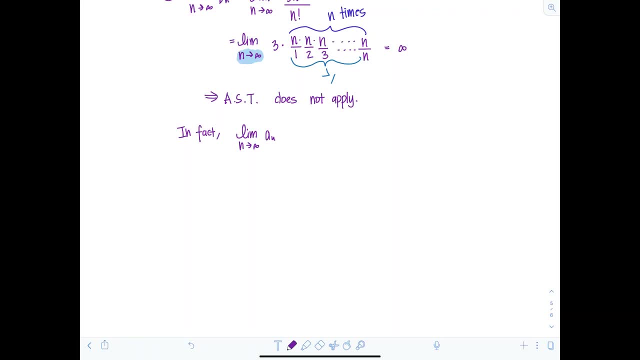 diverges. So I'm looking at the limit as n approaches infinity of a sub n. that's the limit as n approaches infinity. include the alternating part 3n to the n over n factorial. I know it does not exist. Why is that? And all you need to state is that the even terms they're going to approach. 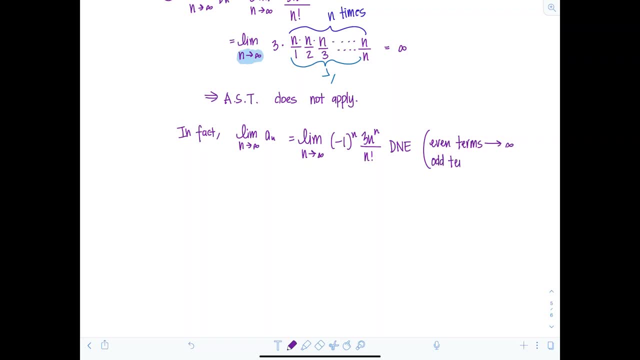 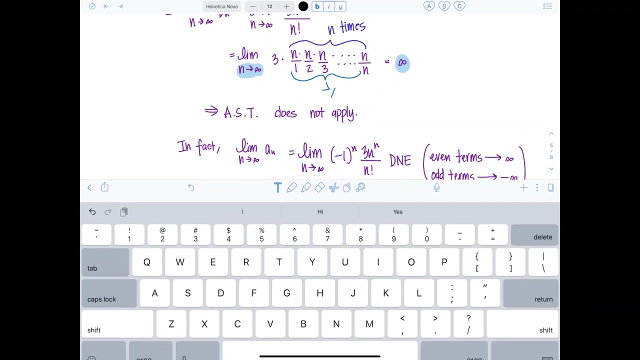 infinity of a sub n. that's the limit. as n approaches infinity, include the alternating part, infinity and the odd terms. they will approach negative infinity, And I'm basing that conclusion on the result from condition 2 failing. So what does this tell me? Well, therefore, 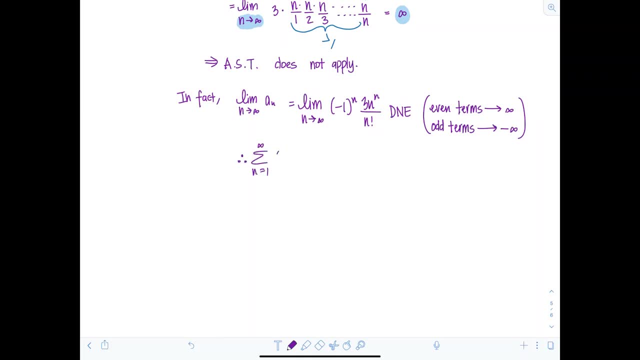 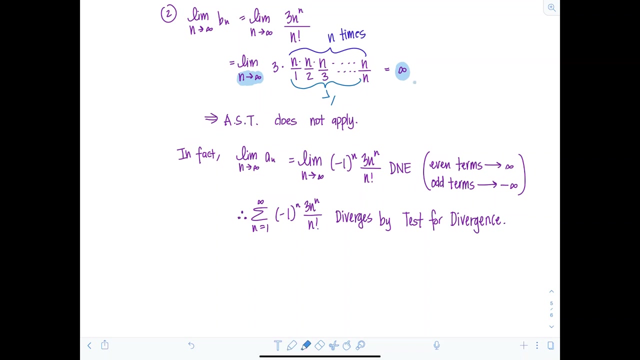 the sum n equals 1 to infinity of negative, 1 to the n times 3n to the n over n factorial diverges by the test for divergence. All right, anytime. this limit here from condition 2 is not 0, you can conclude the test in the same. 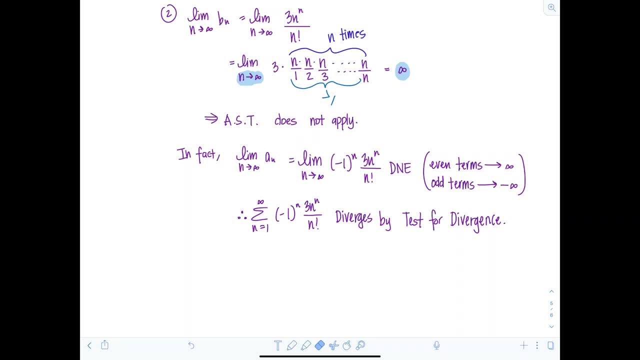 way You could apply the test for divergence. you could say the limit as n approaches infinity of a sub n doesn't exist. and you could say the limit as n approaches infinity of a sub n does not exist because the even terms are going to go to one value, where the odd terms are going to go to the.